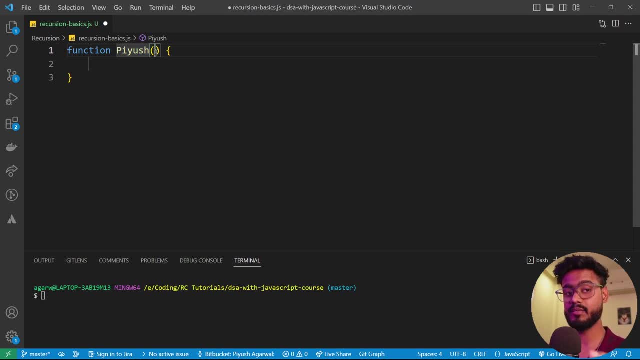 So I'm going to take five functions over here, And each function will represent a single person. So let me write this out real quick, Just like this. So, as seen before, it all started with me, So okay. 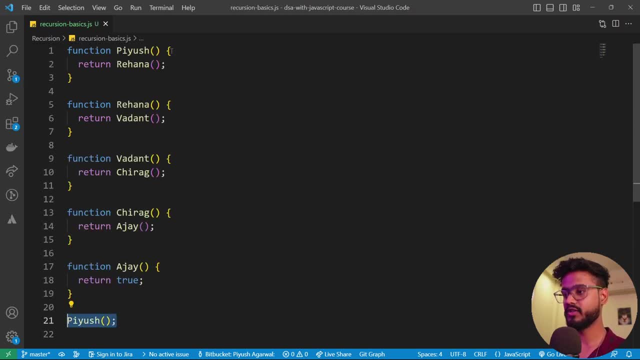 I'm going to call this function over here, Right? So I'm calling Piyush over here And Piyush is calling Rihanna for asking for lunch, Right? But the response of Rihanna is dependent on someone else That is Vedant over here. 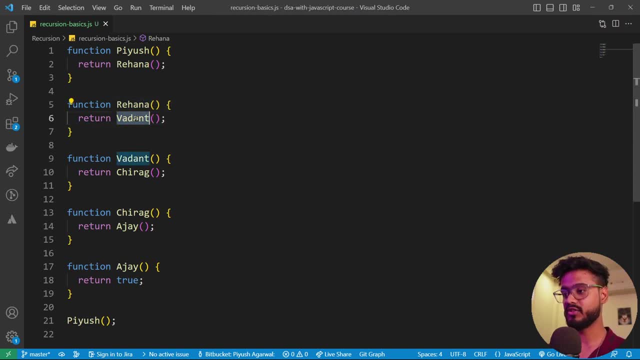 So she is calling Vedant right now, But the response of Vedant is dependent on Chirag And Chirag's response is dependent on Ajay. So, as you can see, these functions are calling some other functions And the response of that particular function is dependent on some other entity or some other function. 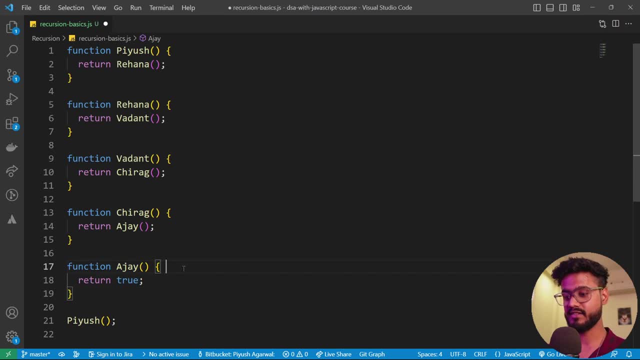 Right, But in this case, Ajay is base case, So this is what we call base case And this is what is responsible for resolving a recursion, As the recursion will keep on going, on, going, on going. So Ajay responds with true. 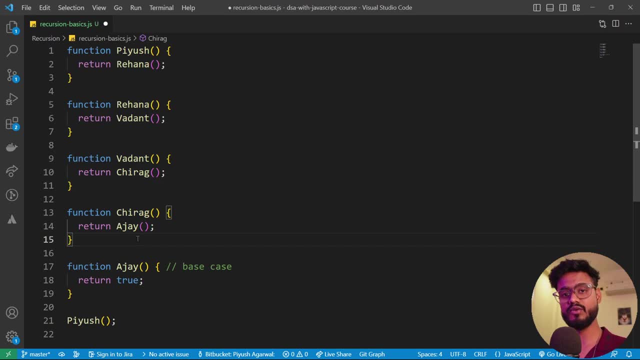 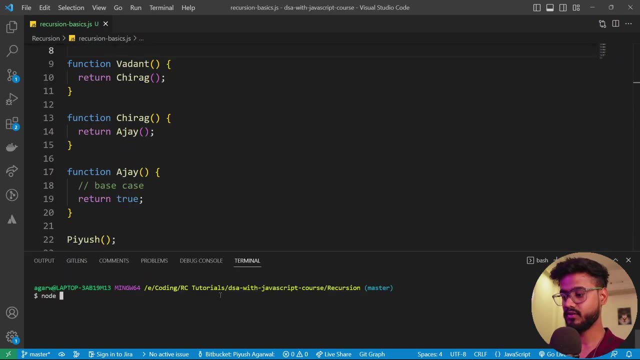 So all of these other functions will also respond with true. If it responded with false, then all of them will respond with false, Right? So if we just try to run this Node- recursion basics- And obviously I haven't console logged this- 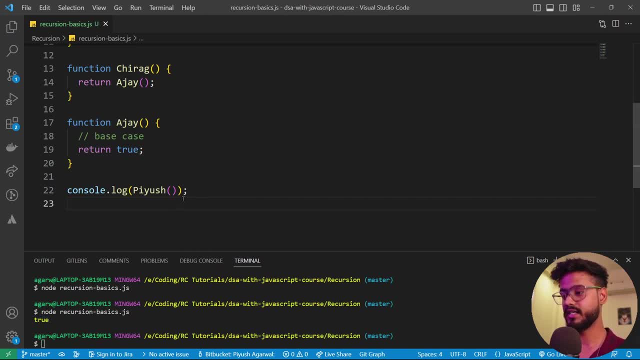 If we try to run this Yep, You're going to see we get true over here. That is, Piyush in the end will return true Because all of the Other functions did return true. But then you will say: how is this related to recursion? 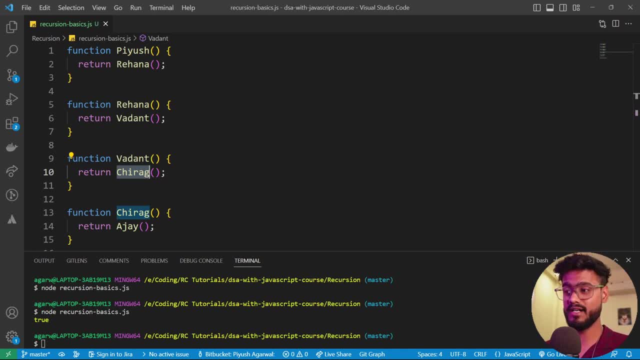 Isn't recursion about a function that keeps on calling itself, But here you have written multiple different functions. Yes, you're right, And this is just a representation to show you how a recursive function will work when we go on to convert this scenario into an actual recursive function. 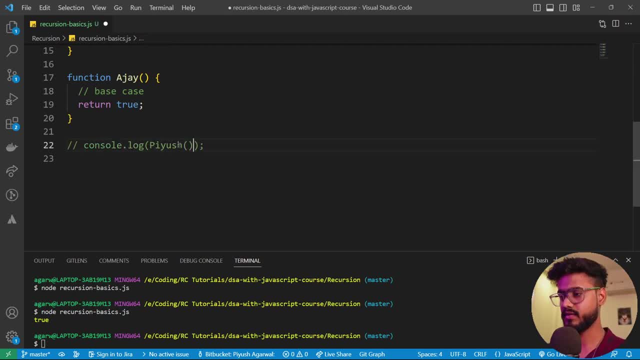 But first let's see how a normal recursion looks like. So comment this out And I'm going to create a function over here called Recursive function, and inside of it I'm just going to say recursive function, because that is what recursion is all about. right, 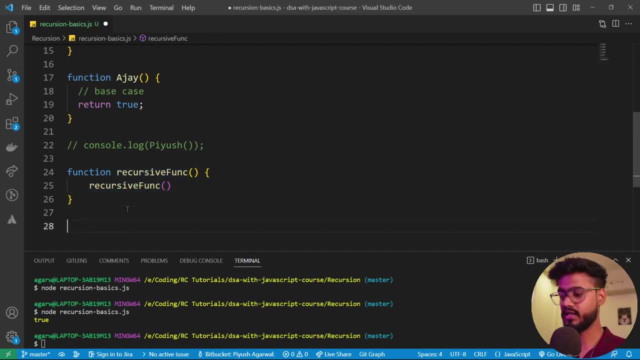 It calls itself like it calls the function. Okay, So I'm just going to call this function once and then this is going to keep on calling itself. Let's just console log it over here. I'm going to say called. Let's see how many times this get called. 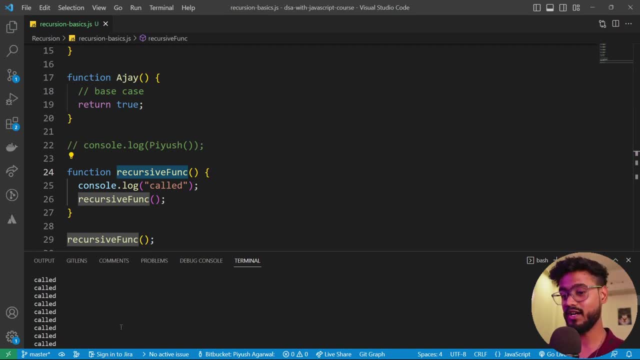 And, as you can see now that we are stuck in an endless loop, that this is being called again and again, and again and again. So this is the. This is the exact reason why we need a base case to stop a recursion. How do you add a base case? 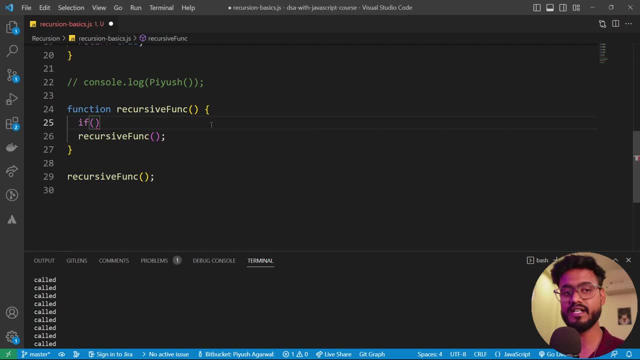 So let's say this is going on right. So to add a base case, we have to add an if condition or any sort of condition. So I will say: if this is true, then return something. right. It can be anything like it can be as one particular condition that breaks this recursion, as this is going to keep on looping forever. 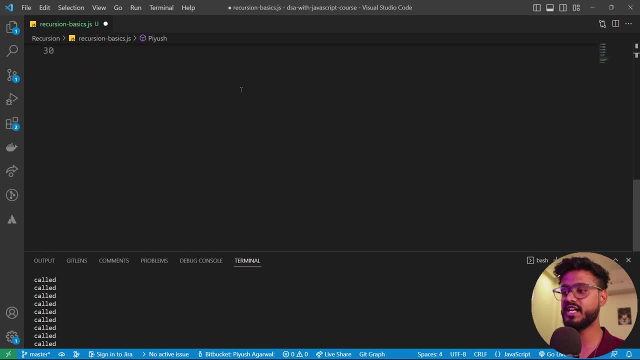 So let's get back to our previous example, This example, And let's try- Let's try- to create it by using a recursive function. So what I'll do is I'll just name this as, let's say, go to lunch, and we're going to start with the first person, right? 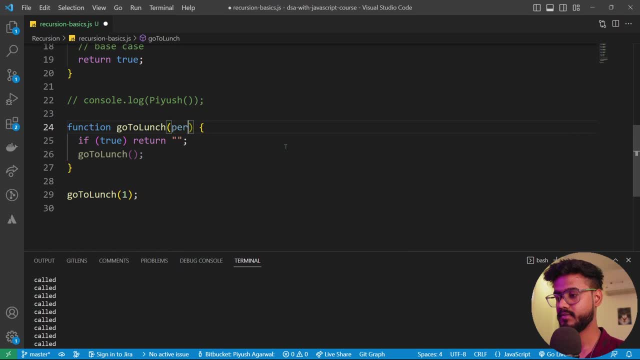 So I'm just going to provide it one over here and I'm going to say so. we have total five people over here, right? As soon as it reaches the fifth person, I'm going to break it. So this is one by default. 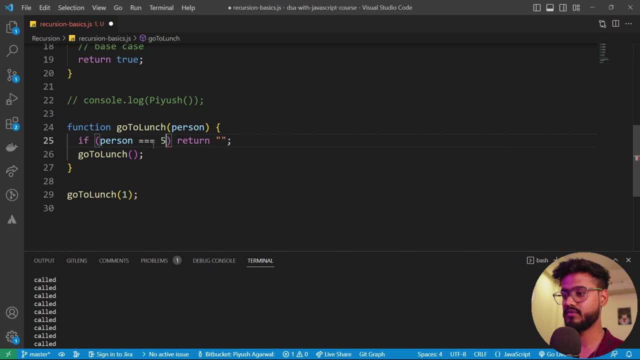 So I will say: if person is equals to five, Then return. true, Else, we're just going to call it with person plus one, because obviously we're going to move to next person, right? And you know, I'm just going to console log it over here. 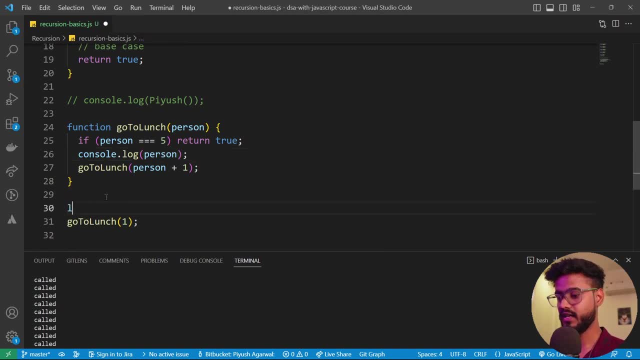 Just the value of percent to see where we are currently, and I'm going to console log this one over here as well. I'll just say outcome to know what's the outcome of all of these calls. And yeah, I think let's try to run this. 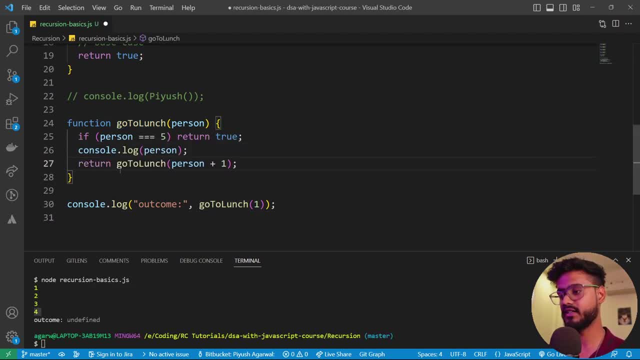 And oops, my bad, I need to return here as well. right, So that it returns the value to the previous functions as well. So now, if I run this, you're going to see first person, second person, third, fourth. 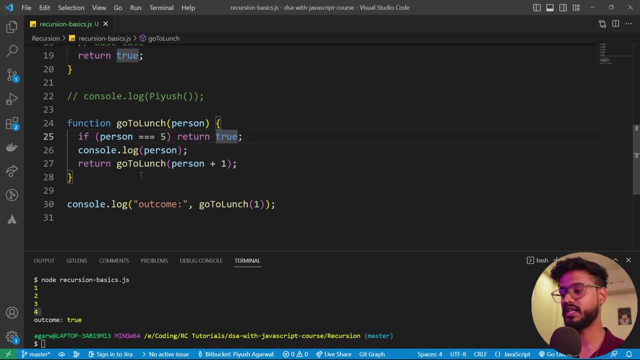 And as soon as it reaches the fifth person, it returns true, so that all other previous functions can also return true. Now I know this might be a little bit hard for you to understand it one go, But don't worry. as we move forward in this video, you're going to get a much more clear. 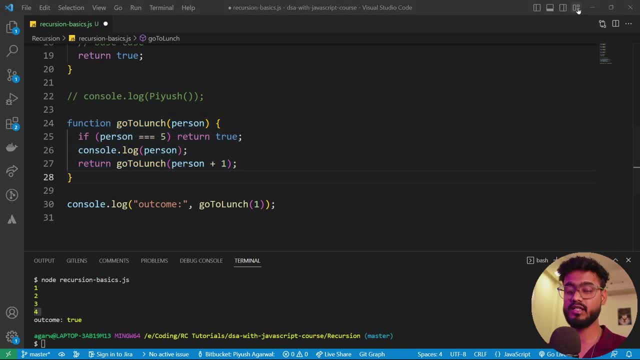 understanding as we discuss more and more example of recursion. Now I know you might be thinking: why do we need recursion in the first place? So recursion is a very important topic when it comes to a lot of algorithms such as tree and graph traversal algorithms. 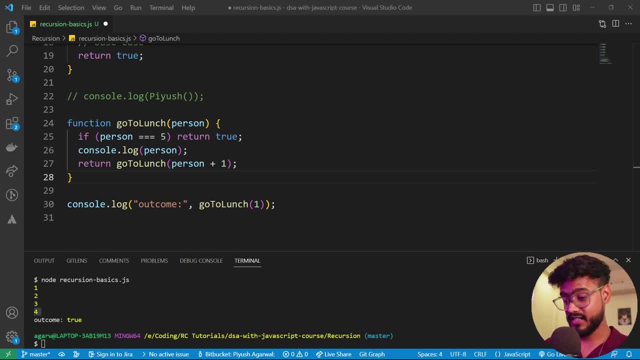 a lot of sorting algorithms, divide and conquer algorithms, backtracking algorithms, dynamic programming and much, much more. So recursion is a very ground level, important topics for what is about to come in this course and data structures and algorithms in general in JavaScript. 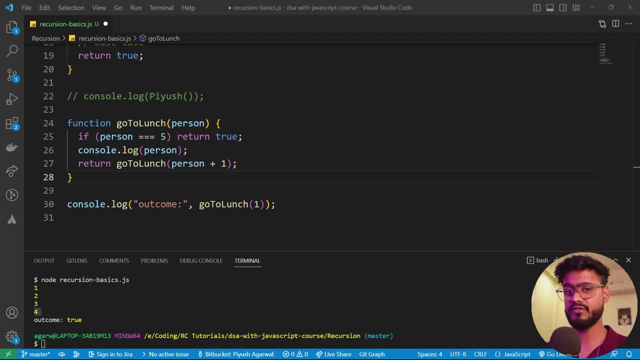 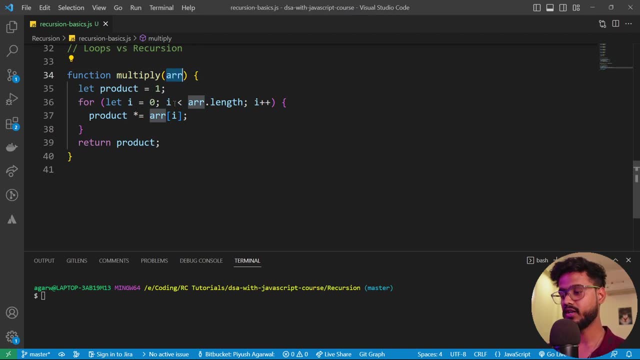 So let's see an example on how you can Convert a function that is written by using for loops into a recursive function. So we have this function over here called multiply, which takes an array, And what it does is it multiplies all of its elements. 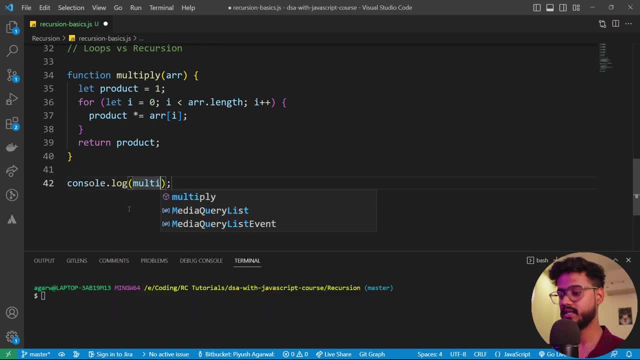 So if I console log multiply And provide it with a simple array, let's say one, two, three, four, Right, and now if I try to run this, you're going to see we get twenty four. so four multiplied by three, twelve, twelve to the twenty four. 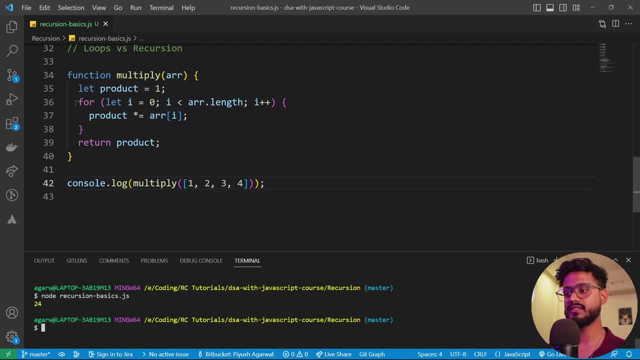 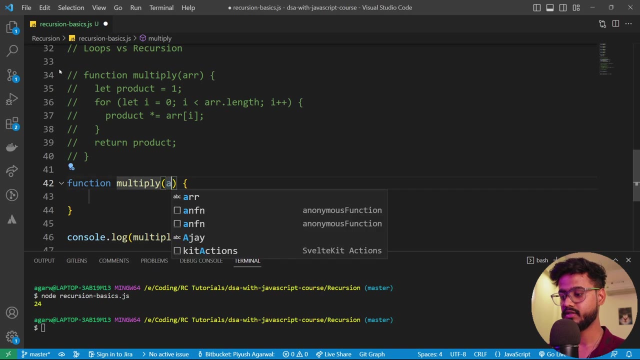 Into one is one, So we get twenty four over here. Now we are using simple for loop over here and multiplying each element with another. So how do we convert it into a recursive function? OK, let's comment this one out What I'm going to do. I'm going to write another function called multiply. 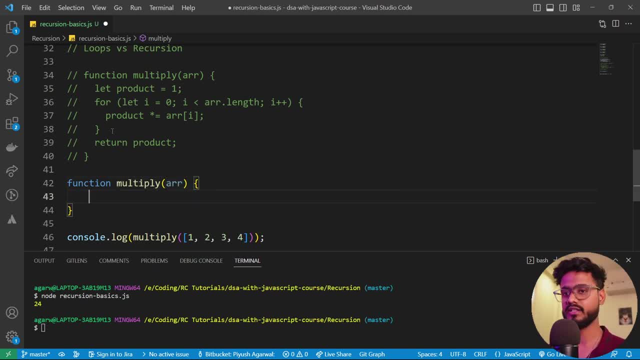 Which again will take an array. And now what are we supposed to do over here? So, in this for loop, what we were doing is we're taking and global state called product, which was by default one, And for each iteration We were multiplying every single element into that global result. 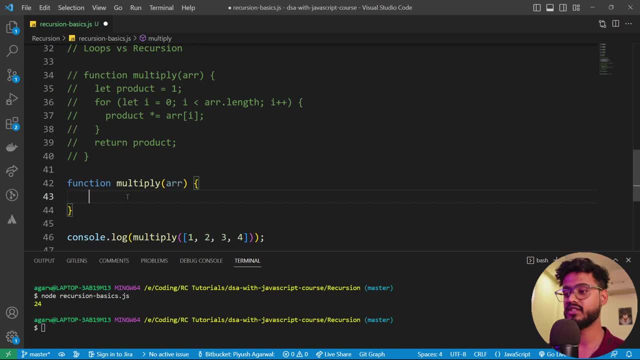 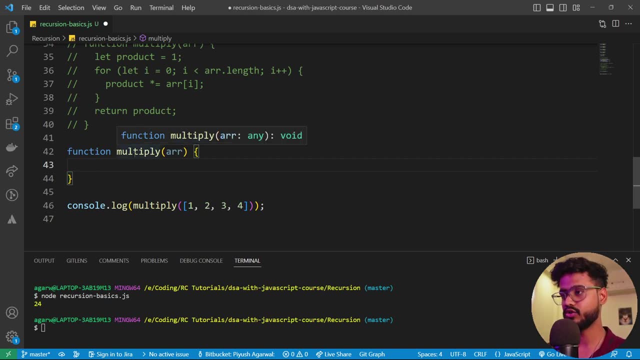 But in recursion we don't have any global state as such. So what we can do is we can divide this problem into small, small parts and then we can multiply them all together. So let me show you. So what we can do is we can say return and we can take the current element. that is the last element or the first element. 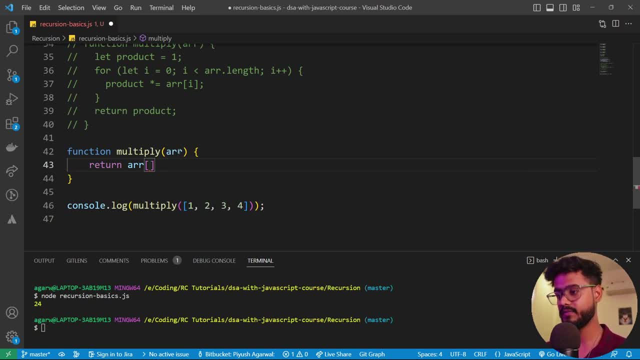 So I'm going to take the last element, which in this case, is going to be array dot length minus one. So I've taken that, I've taken this last element over here, and what I'm going to do? I'm going to multiply it with the rest of the result, because that is what we're supposed to do, right? 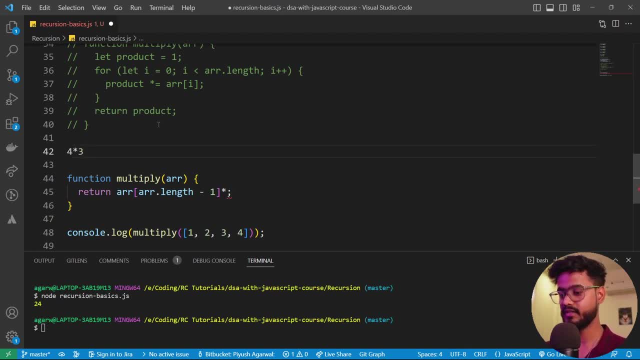 If we have one, two, three, four as an array, we're supposed to do four multiply by three, multiply by two, multiply by one right. So in this case we have accessed four over here. Now how do we access three? 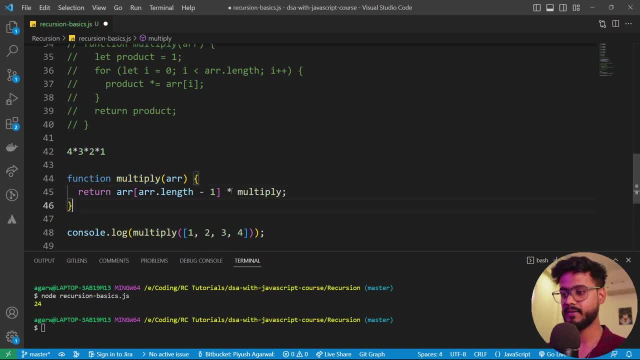 What we can do is we can simply call this multiply function And we can provide it array and remove one, And from the array array dot slice zero comma. array dot length minus one. But wait, there's going to be one moment where this array becomes empty, right. 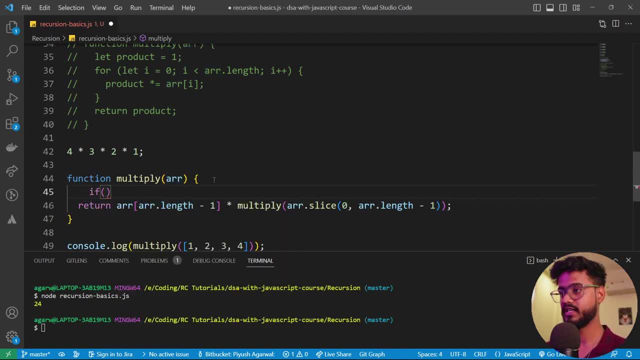 The length of this array becomes empty. So I'm going to put an if condition over here. If array dot length is less than or equal to zero, Then I'm going to return one, because there's nothing to multiply over here, right? So I'm just going to return one else. 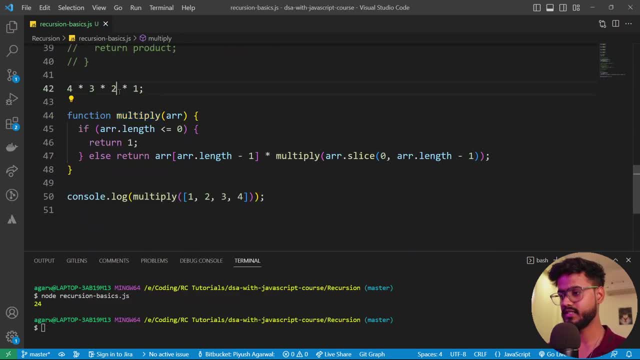 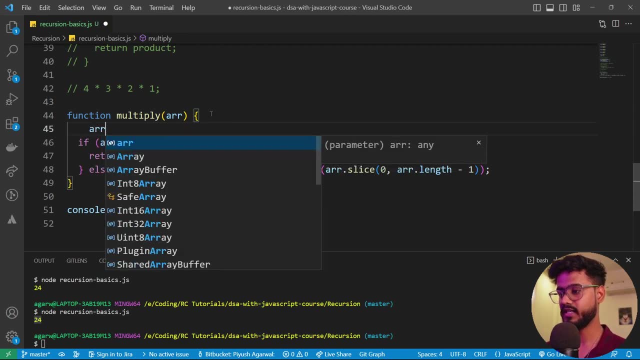 We're going to do this. I think this should work. Let's, let's find out. Yep, You see we get 24 over here, So let's deep dive what's going on over here. If right at the beginning I try to console log the array, you're going to see. 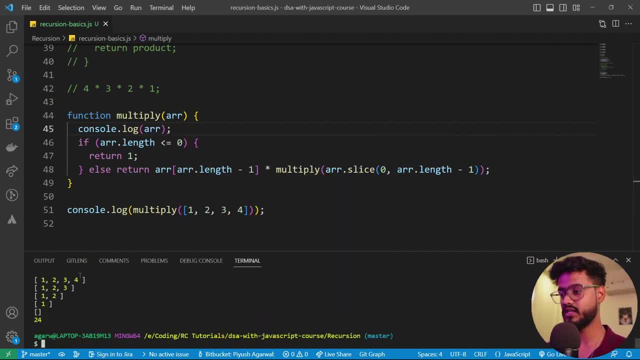 And now, if I try to run this, you're going to see first we have one, two, three, four. In the first call we have one, two, three, four. Then in the second call, since the array dot length is not equal to or less than zero, 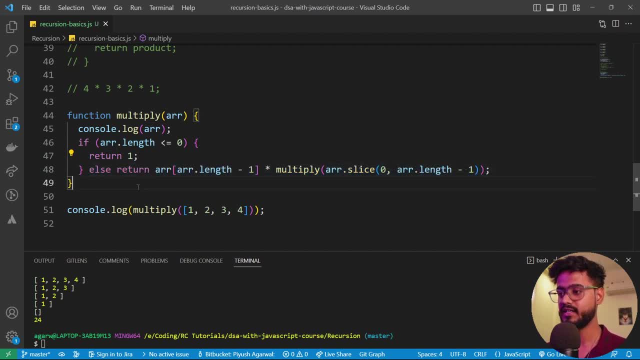 So we're going to go to this line over here, We're going to take the current element, that is four, and let me just explain with this. So we have, we currently have four over here. four multiplied by this multiply with: array dot slice zero, comma. array dot length minus one, that is zero to three. 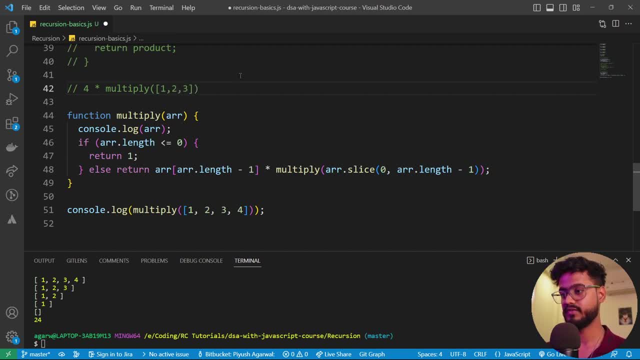 So this will be one comma two, comma three. This is what we're going to call. So now we have multiply with one comma two comma three. again, Length is not equal to or less than zero, So we're going to go to this statement again. 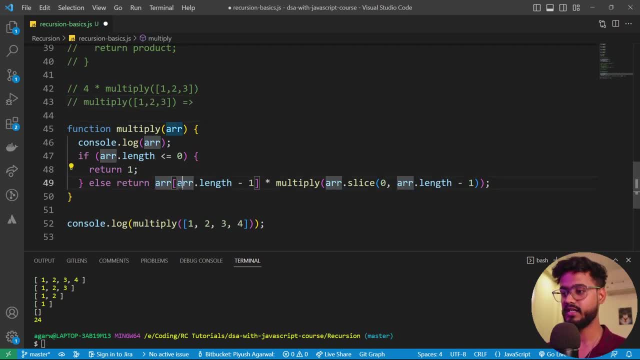 Now for this function call. what will be the scenario? It will be array, array dot length minus one, which is in this case three. So I will say three multiplied by this multiply function. But again we're going to slice to array length minus one. 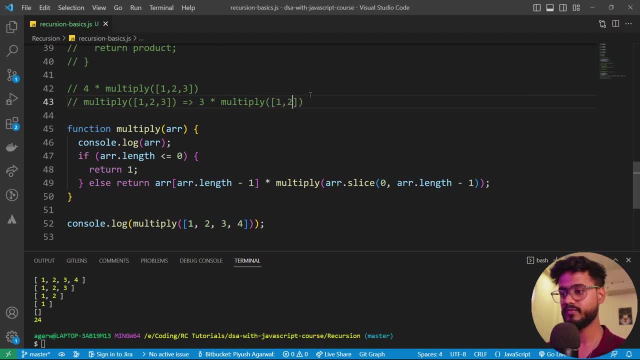 So now this will be one comma, two, Right? So again, this will evaluate this one. First of all, let me just take this and replace it over here. So now we are at over here, Now again, it's going to take the last element, that is, two, and multiply it by multiply. 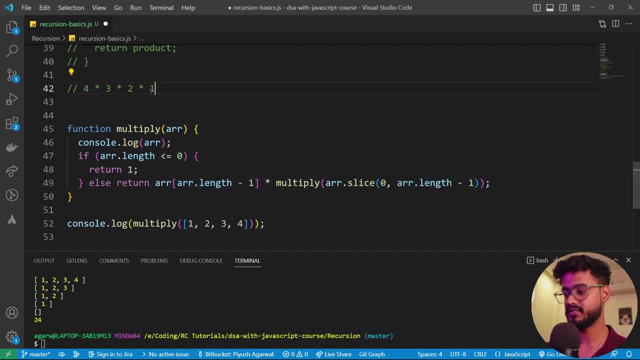 And now array will have one, just like that. And again, when we call this, then we will have one, and then we reach the base case, which is if array's length is less than or equal to zero, which is going to be again. 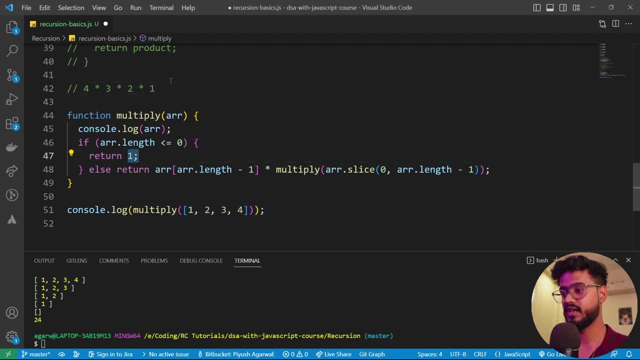 something like one, Right? So then we're going to return one, and now we're going to return each and every value for this recursion and we're going to multiply them, all of them together, Right? So that is when we will get our final output of 24.. 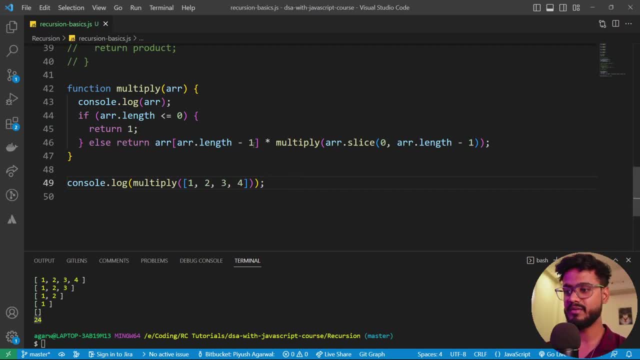 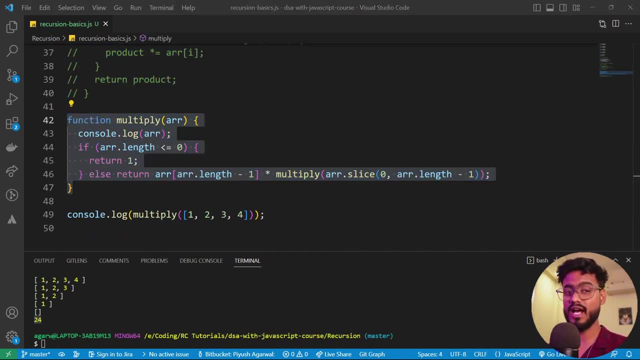 So that is how a basic recursion works. Now you might be thinking which one is better. is the looping approach better or the recursive approach better? So, to be honest, there's no right or wrong answer to that. It's up to you and depends on the particular problem that you're solving. 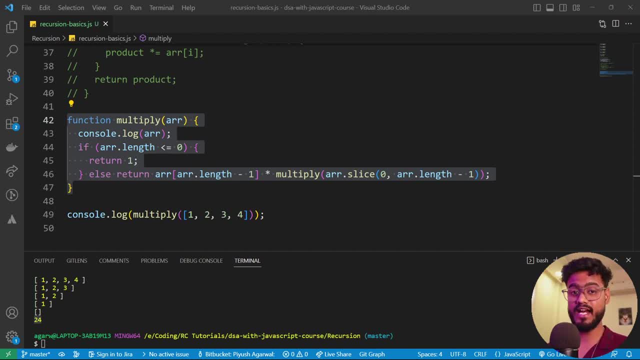 When it comes to looping, When it comes to writing code, you have to make sure that it's easy and understandable to read, and recursion can sometimes result in a shorter and more simpler code. So that is why we emphasize on using recursion a lot. 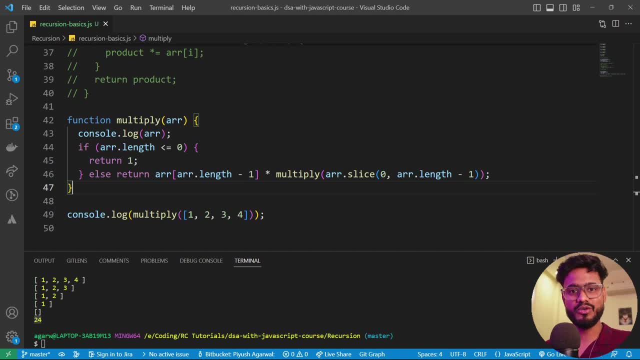 And that is why I have a question to ask you: Why did a programmer go broke? Because he kept on calling himself and his bank account reached the base case of value, zero. You know, because he kept on calling himself and each version of him spent that money. 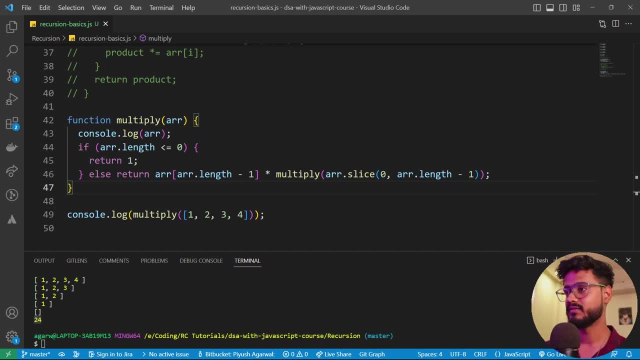 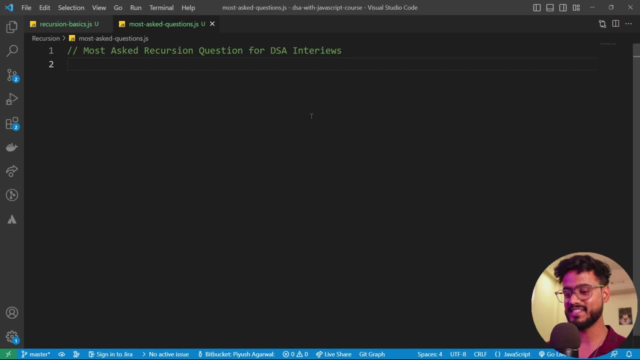 So you know there was a one point it reached, nevermind. Alright, now let's see one of the most. alright, now let's see the most asked recursion questions that are asked during our DSA interviews. So the first one will be factorial of n. 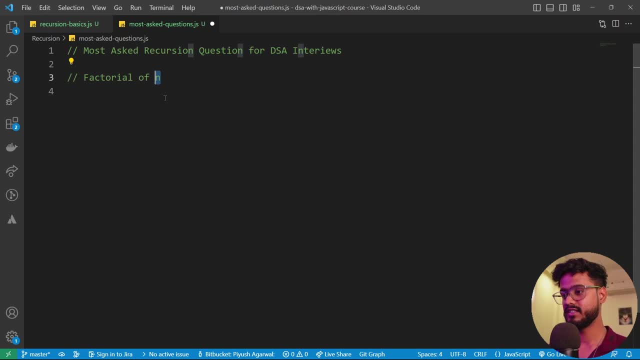 So what is this factorial all about? So when we have a number, which in this case will be n, so let's say n equals five, So factorial of five will be five into four, into three, into two. So I'm going to get a function called factorial which will take n as an input. 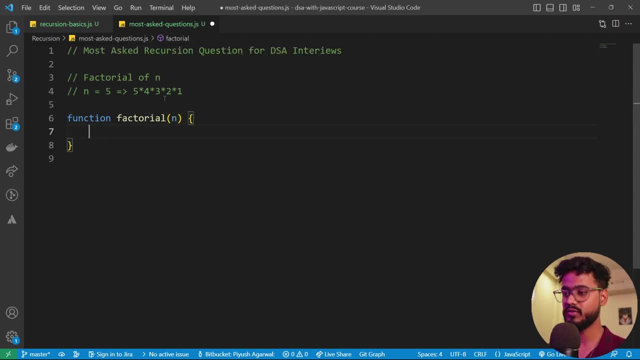 And now we're supposed to return the factorial of this function. So I would highly recommend you to go and try this question yourself first, because it's very similar to the previous question that we just did. So, yeah, pause the video and try this question yourself, and then continue with this video. 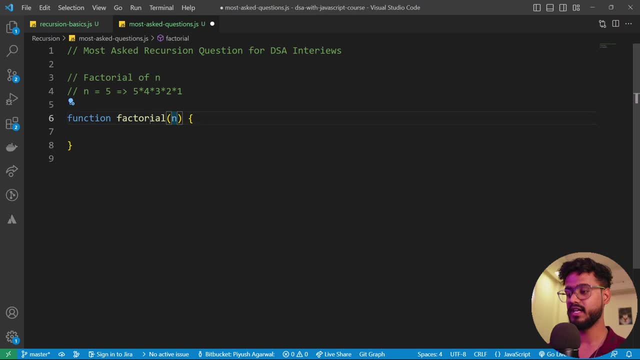 So, okay, I hope you've done this question. If not, let's continue. We have a function called factorial and we're taking n as an input. So if we say console, So log factorial, and let's say we take five as an input, right? 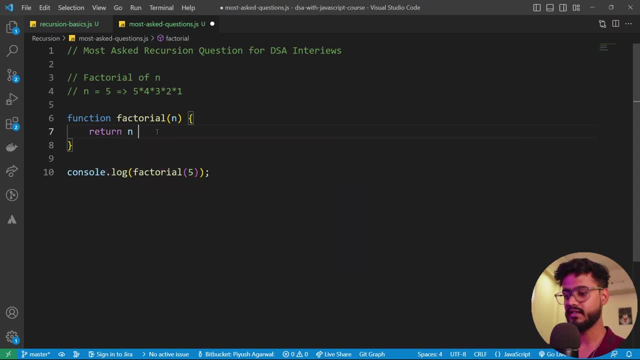 Now, right now we have five over here. So I'm going to say return n into. so, as you can see, whatever the value of the number is, that is multiplied first, right? I mean, that is the part of our calculation. So what I'm going to do is I'm going to say n multiplied by whatever comes next, right? 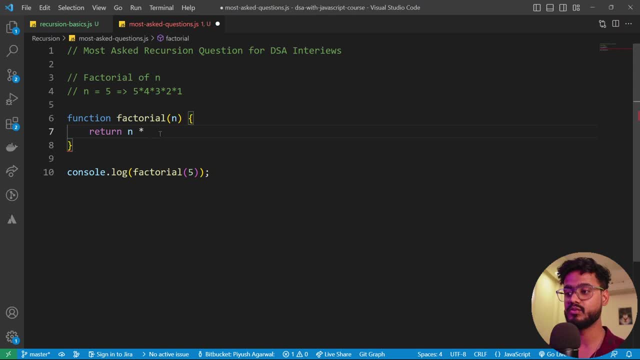 Now, what are we supposed to do? we're supposed to do n minus one. So can I just not take this function Okay, And call it again with n minus one, simple right. So now it's going to be five into n minus one, which is going to be four into three. 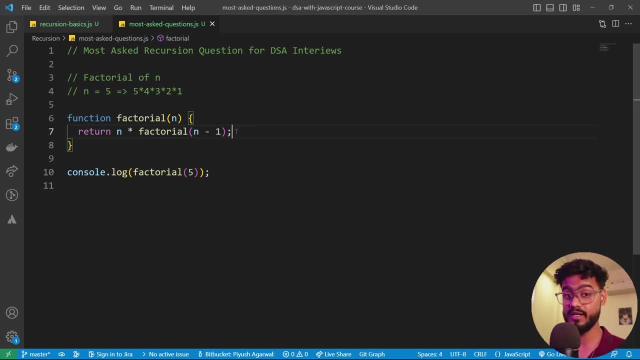 into two, into one, But again, we have to take care of our base case. So what can be the base case in this? So, as soon as this reaches the value of zero, we're going to return one, because it's not going to go further, any further than that. 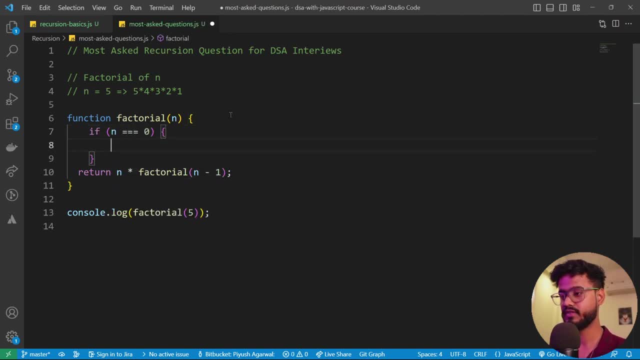 So I'm just going to simply say: if n is equal to zero, Then just return one, Okay, Because if you multiply anything by one it won't make any difference, right? So that is why I'm returning one over here. else you can return n into factorial n minus. 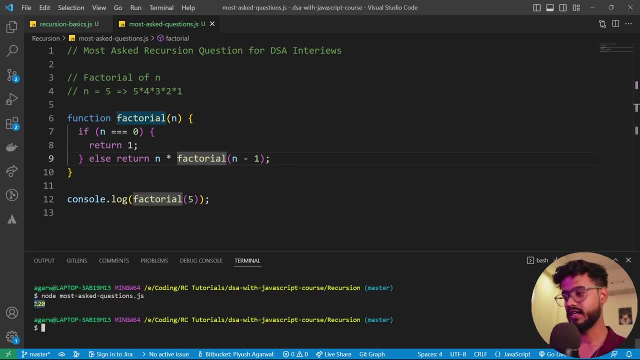 one. Cool, Let's try to run this. All right, we get 120 over here. Hmm, Let's see. So, five multiplied by 420 into 360, into two, 120.. Okay, fine, We have 120 over here and that is what we're supposed to get. 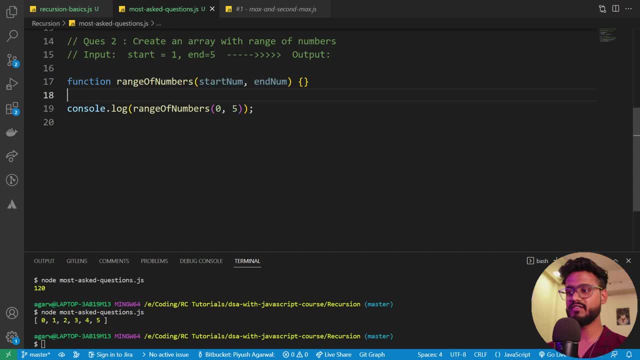 Awesome. Now the next question is the range of numbers. So in this question we're supposed to create an array with the range of the provided number. So we're going to get one start variable and other the end variable. So, as you can see, we have this start num and end num and we are calling this range. 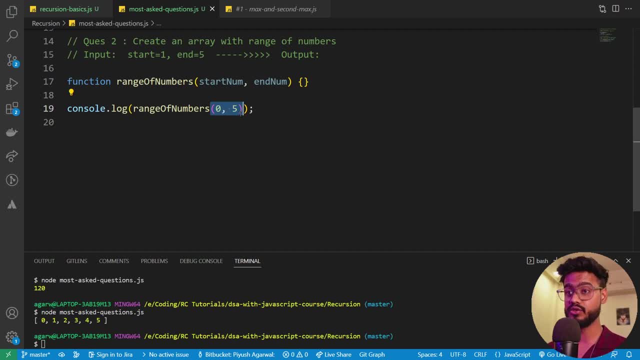 of number from zero to five, and you have to use recursion to do this. So, again, I would highly recommend you to solve this question yourself first and then move on with this video. So I hope you are able to do this. Let's see how we can do it. 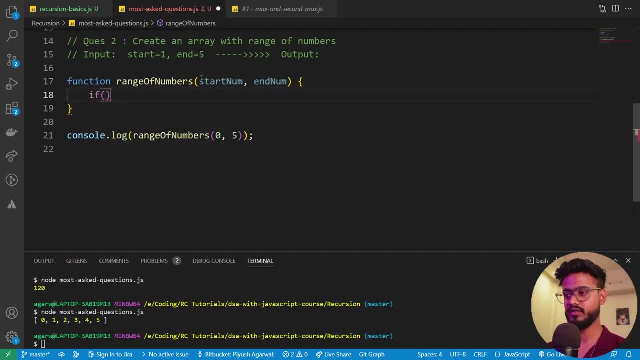 So first of all we're going to check the base case first. So obviously the start number has to be less than n number. right to generate it from start to end. So simple. We're just going to use our common sense and say: if n num is less than start num, then 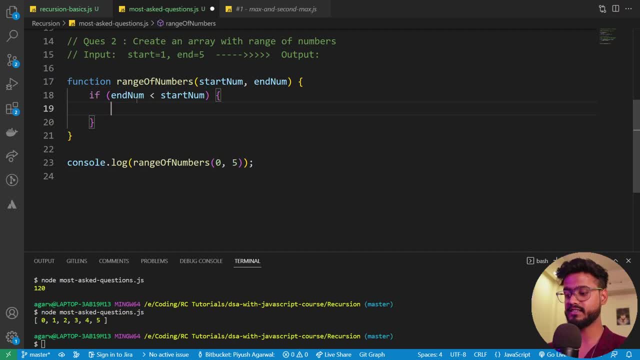 it makes no sense to continue. So this is going to be our base case. If that's the case, then I'm going to simply return an empty array, because there is no chance that we can just generate another array, right else. What we can do is we're going to say const numbers variable and I'm going to say range. 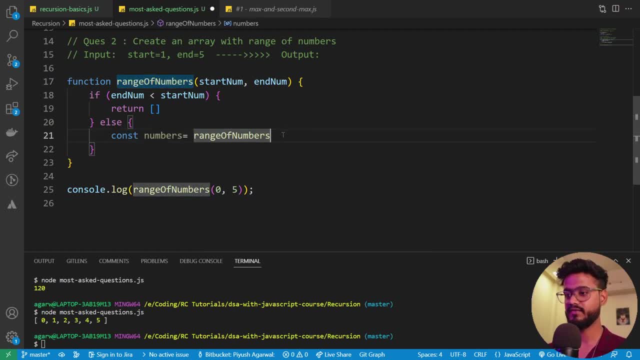 Okay, Of numbers, We're going to call this function again with start number and n number minus one. So with each iteration, with each recursive call, So if we have n number as five, so it will be four, then three, then two, then one, then 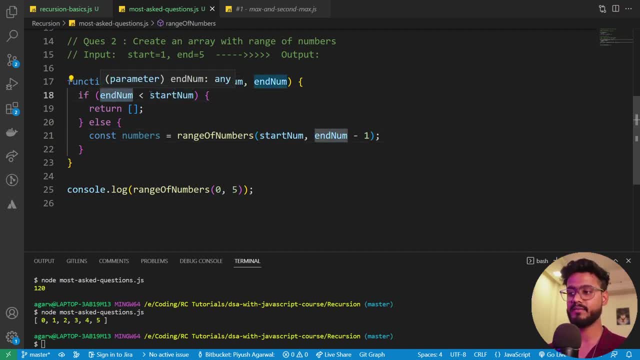 eventually zero. So it will go below start number right, And as soon as that happens, it's going to return us an empty array. And since this is going to return us an array, over here This numbers will be an array. So I will simply say numbers, dot, push and push the current element, that is the end number. 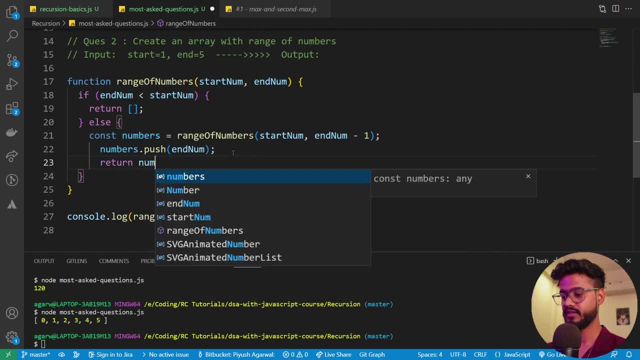 So n num over here and I'm just going to return numbers. Let's try to understand what's going on over here. So if I try to try run this, so first of all we have range of numbers with zero comma five. 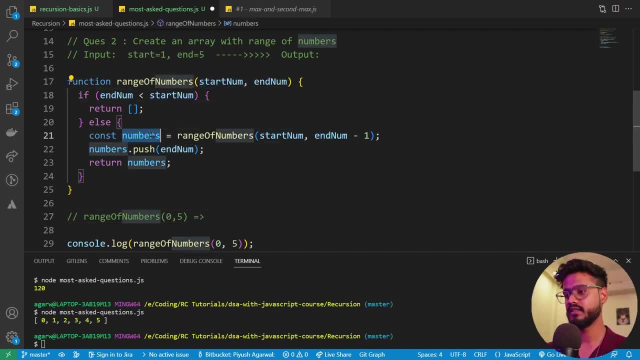 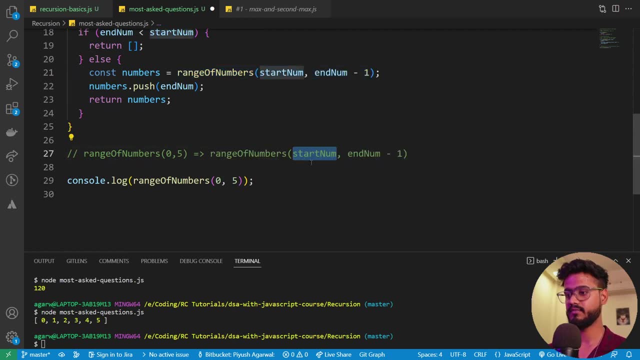 Now, in this case, the n num is not less than start num. yeah, obviously, And over here we are calling this function again first. So, okay, fine, We're going to call this function again: start num, which is going to be zero. 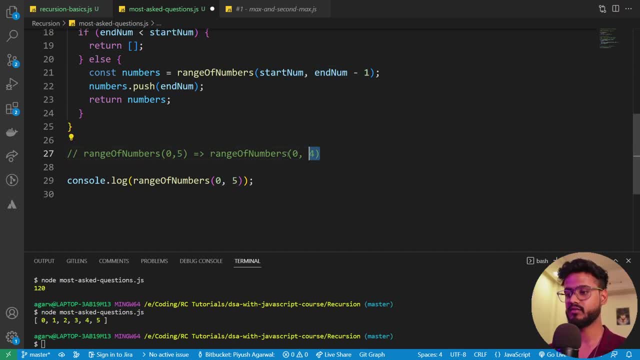 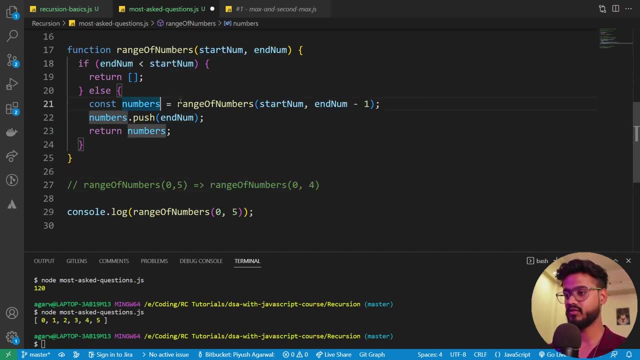 And n num will be four in this case. first it was five, then it was four, Then again it's going to go back, So n num less than start num. no, that's not the case. So again it's going to come back over here. it's going to call this function again. fine. 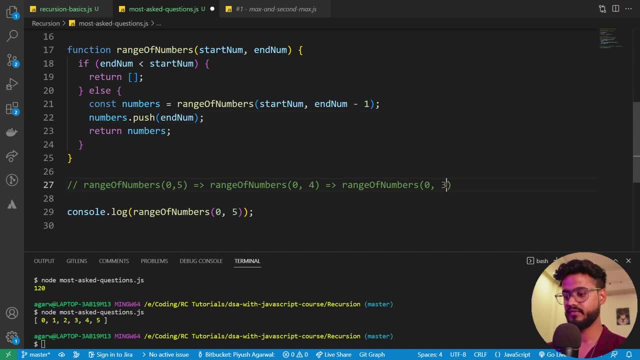 I'm going to call this function again, but this time it's going to be zero comma three. Similarly, it's going to be zero comma two, And then in the end, it's going to be zero comma one. Okay, Let me just write all of these in separate lines. 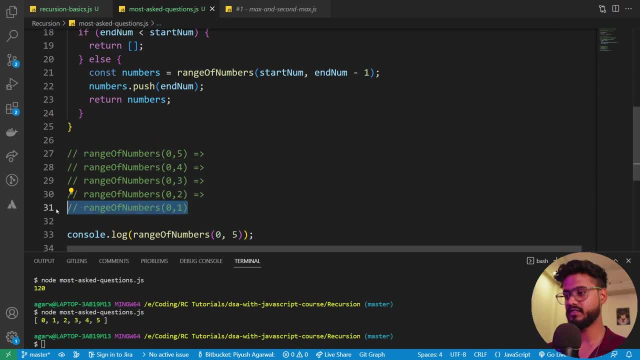 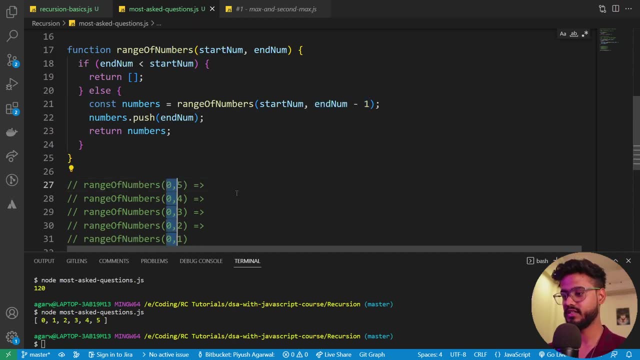 All right, Cool, I think it's clear up until this point. Now, after this, again, it's going to call with start num and n num minus. my bad, this is not zero, This is one actually. Yeah, Sorry for that. 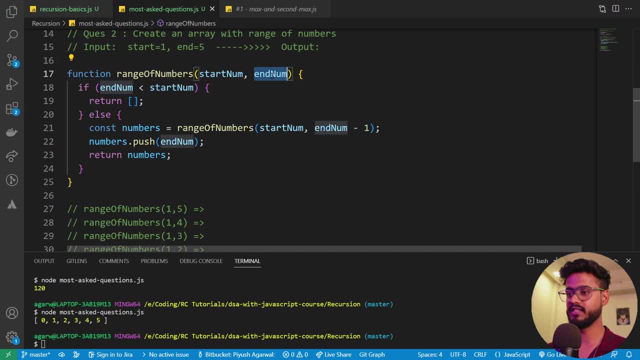 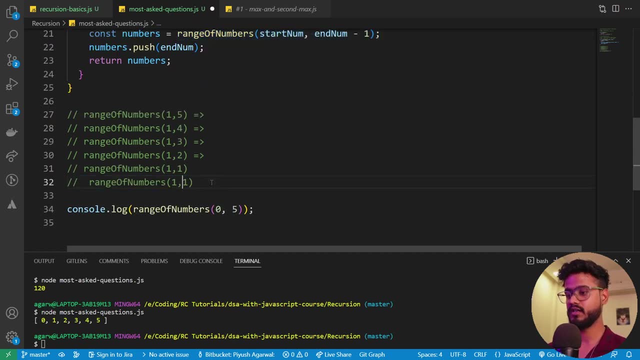 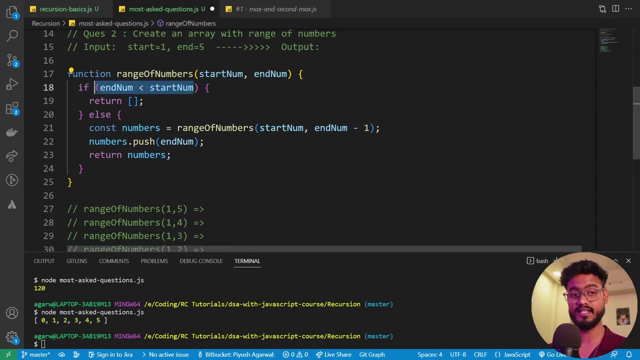 Now, after this iteration, it's going to go over here with one and one, and okay, this is still a satisfies the condition, but in this case it will be one comma zero. Right Now. in this case, what's going to happen? it's going to satisfy our base case. 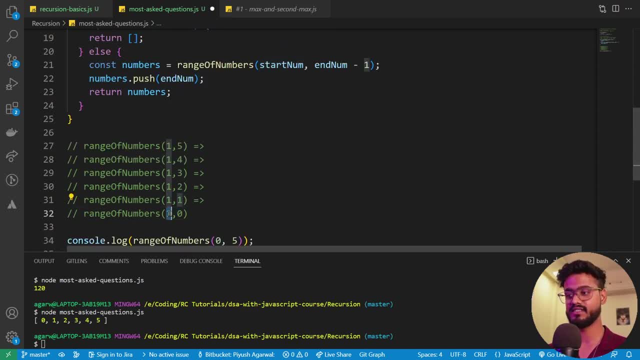 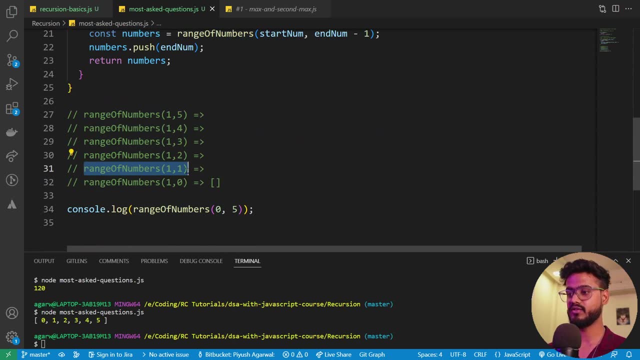 So n number is less than start number. It's zero less than one. Fine, So what we're going to do? we're going to return empty array. Fine, In this scenario, now we get an empty array in this numbers over here. 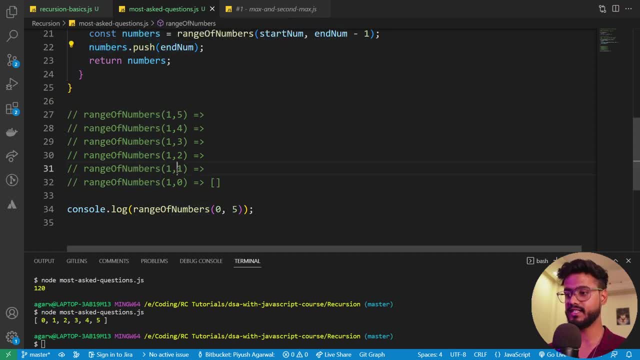 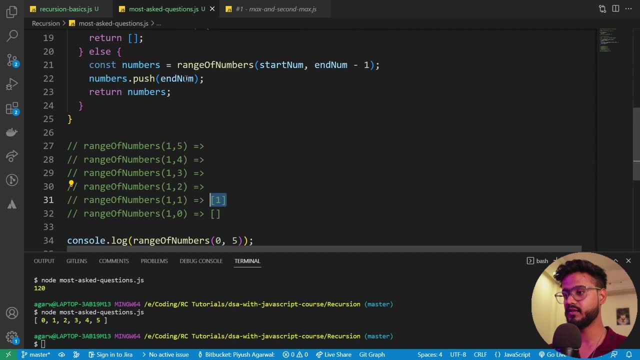 So we can do numbers dot, push n num. So in this case, n num was one, So we just pushed one over here, right, Cool? So we get one over here and then we're going to return numbers, simple. So numbers, in this case, is this one array. 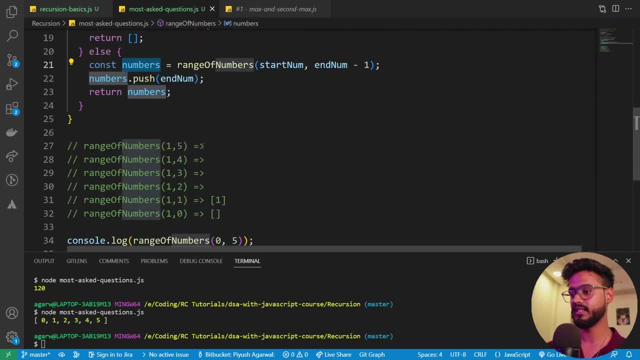 Now we're going to go to this case. Now, in this case, we get in numbers, this array with value one. Now, after this, we're going to say number dot, push n num. Now, in this case, n num was two. 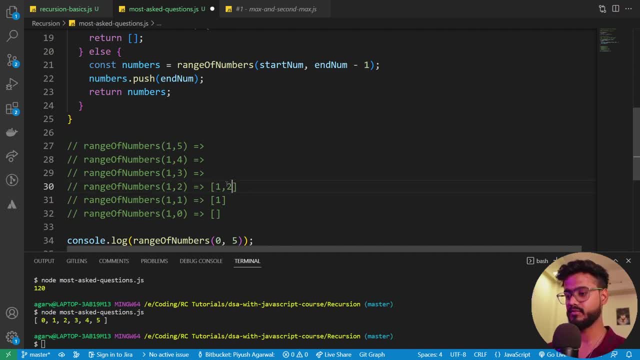 So I will say one and I'm going to push two over here. Simple Again. it's going to return numbers And in this case n num is three. n num is three. So I will say one comma, two comma three. 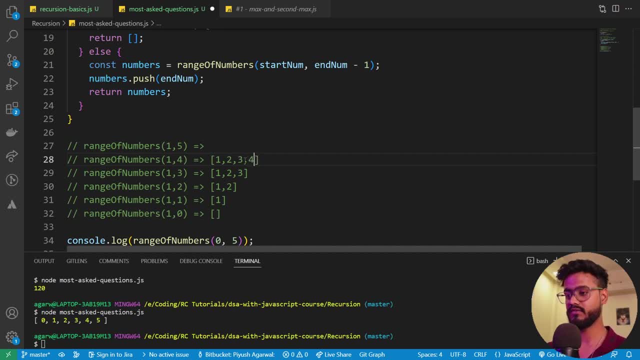 Similarly, in this case n num is four. one comma three comma four. In this case it's five. one comma three comma four comma five. So you see how this bottom up approach worked. We went to the very end of the array and then it returned us with an empty array. 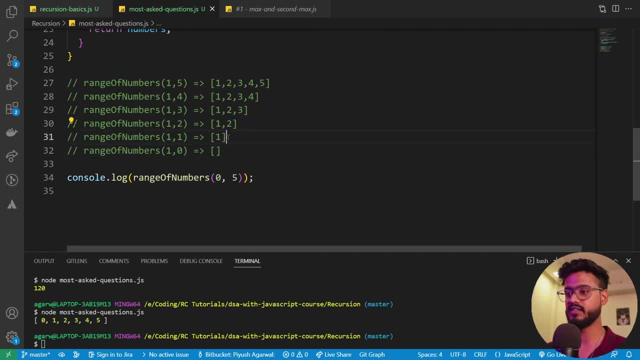 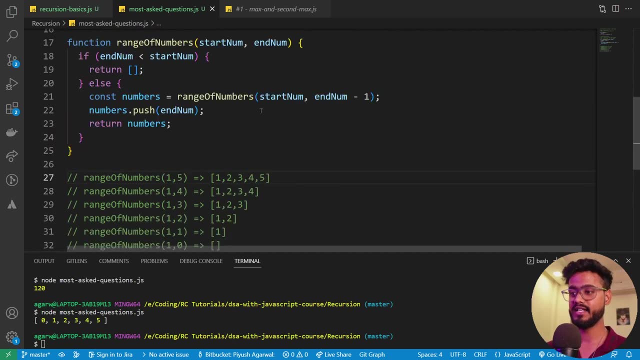 And then we started adding elements to it in a reverse manner. So we first added one, then two, then three, then four, then five. So this is the beauty of recursion: How simple it gets. while writing code with recursion, I know it might be a little bit complex, but with time, as you would have written a lot- 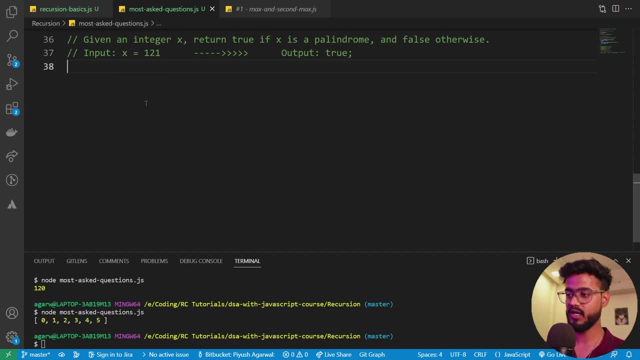 of recursive code. you're going to understand this very easily Now in our next question. we are given an integer, x, and we are supposed to return true if x is a palindrome and false if it's not a palindrome. So what is a palindrome? 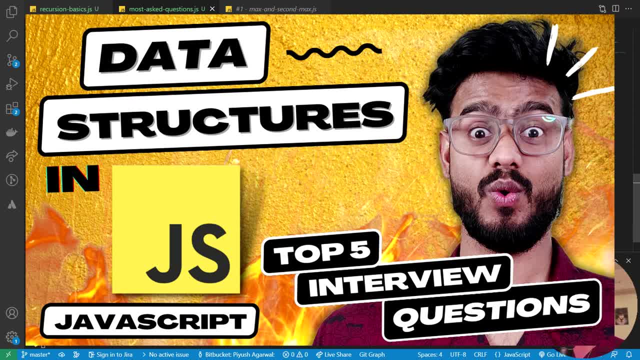 So I've explained this question in a much in depth in this video right over here, So I'm going to play that clip over here for you to understand. So palindrome number is a number which reads exactly the same, So I'm going to play that clip over here for you to understand. 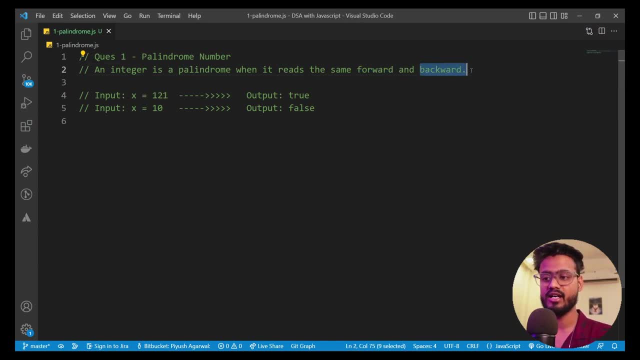 So palindrome number is a number which reads exactly the same. So I'm going to play that clip over here for you to understand. So palindrome number is a number which reads exactly the same when you read it forward or backward. So if this is 121, so if you reverse the number 121, so it's exactly the same as it was forward. 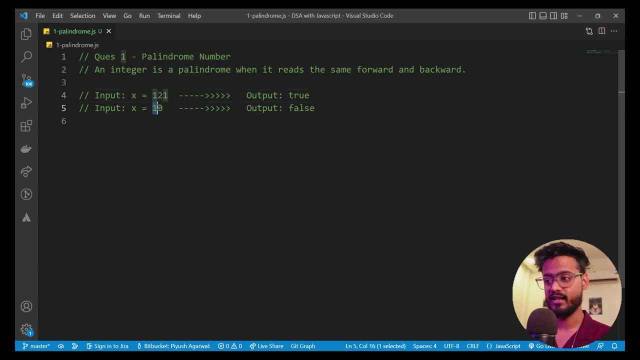 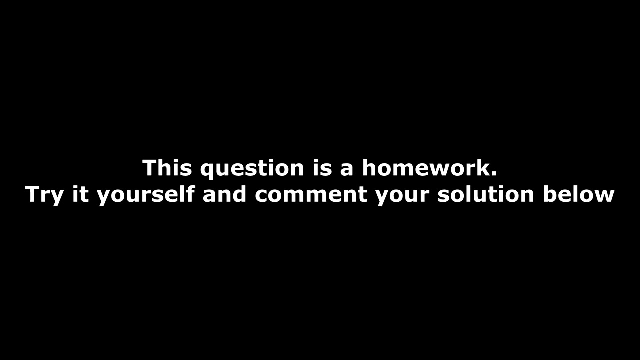 as well as backwards, but that is not the case with 10.. So if you read 10, it's one zero, but if you read it in reverse manner, it's zero one. Therefore, in this case, output will be false, but in the first case, output will be true. 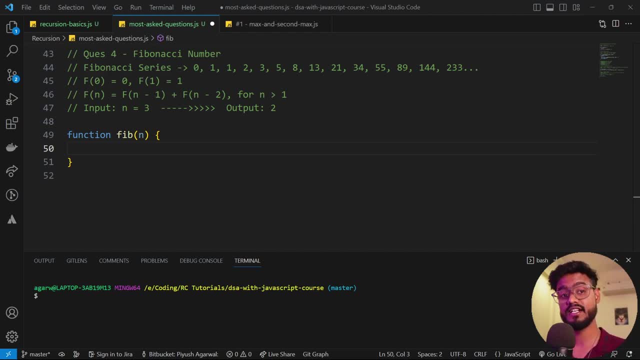 So up until this point, what we were doing was more of example of linear recursion, that is, recursion in one single line. But with this question, this Fibonacci numbers question over here, we're going to see an example of recursion where multiple recursive calls are being made at once. 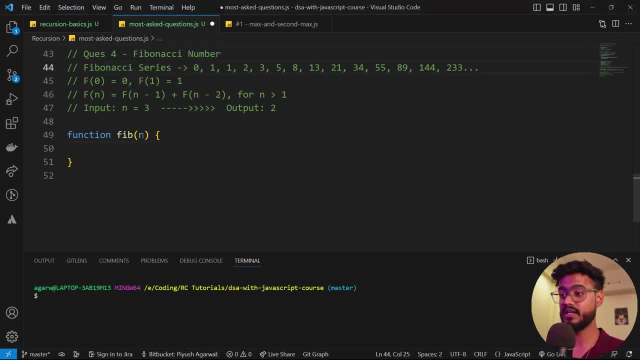 So what is a Fibonacci number? So in Fibonacci number we're given a number n which, let's say in this case, is five, right? So how does this Fibonacci series works? So we start with two numbers- zero and one- Now to get the third number. 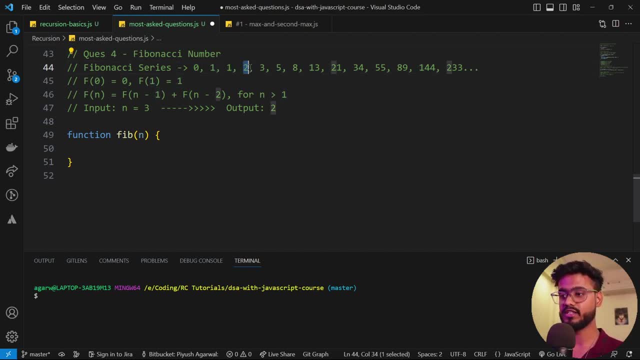 We add zero and one and we get one. Now to get fourth number, we add previous two numbers, That is one and one, two. Now to get fifth number, we add third and fourth number and so on, And as you can see over here, to get F of n, we're supposed to add F of n minus one plus. 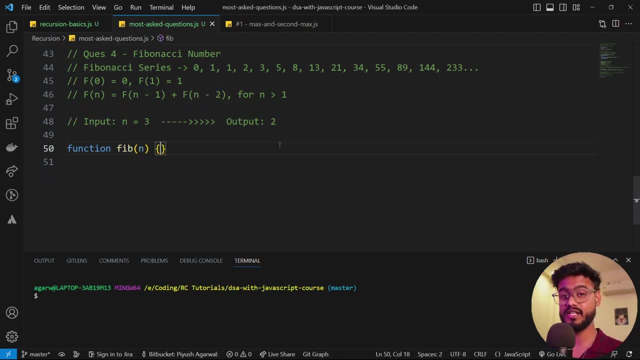 F of n minus two And, trust me, this is a very frequently asked question when it comes to data structures and algorithms interviews, when the interviewer is looking to ask you a question regarding recursion. So let's, before jumping into the code, let's understand how this will visually look. 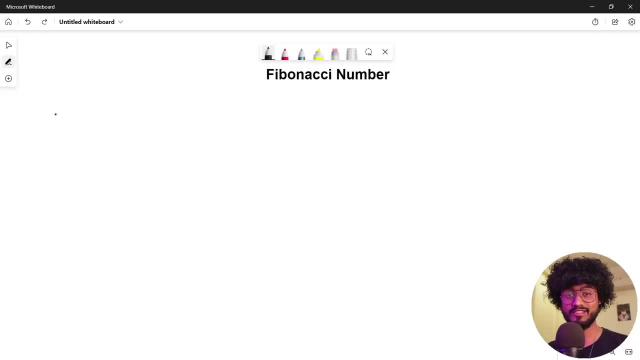 Oh, no, no, no. you're not going to explain this algorithm when Algo Agarwal is here, because people would like to see this algorithm explained visually, and that too from Algo Agarwal. So let's get it. Let me explain you Fibonacci number. how to do Fibonacci number by using recursion in. 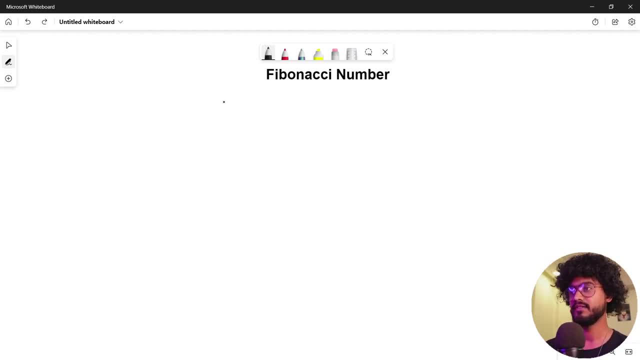 the most easiest way possible. So let's see what is a Fibonacci number. As explained, Fibonacci number can look something like this: So if we want to calculate what's the Fibonacci number for five, So okay, Fibonacci numbers always look something like this: 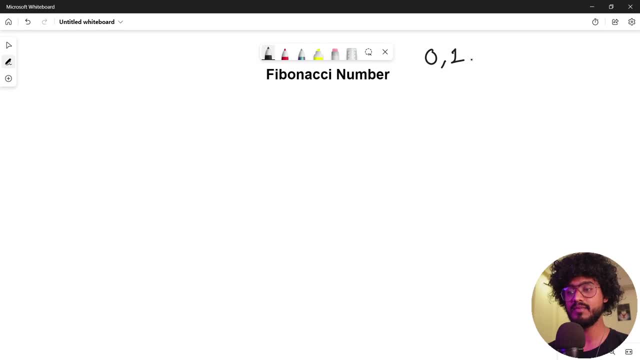 It starts from zero and one, And to calculate the next numbers we have to add the previous two. So zero plus one equals one. fourth number will be one plus one, two, two plus one, three, three plus two, five and so on. 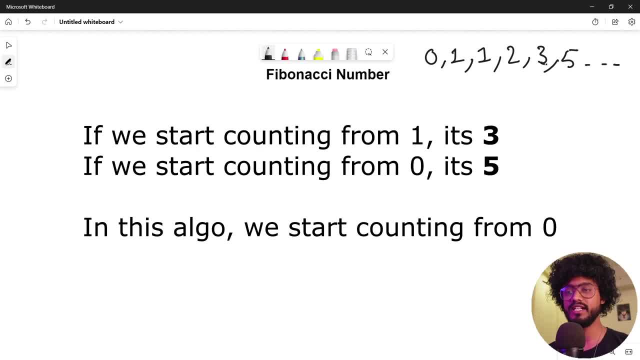 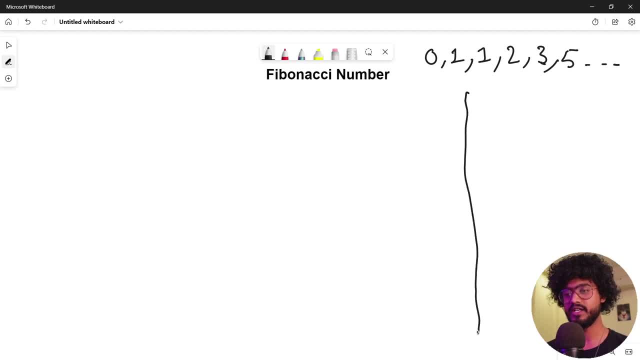 So the fifth number will be 12345.. So three will be the final output when the input is five. All right, So let's see what are the steps that we are going to take to explain this. So let's say we have a function called 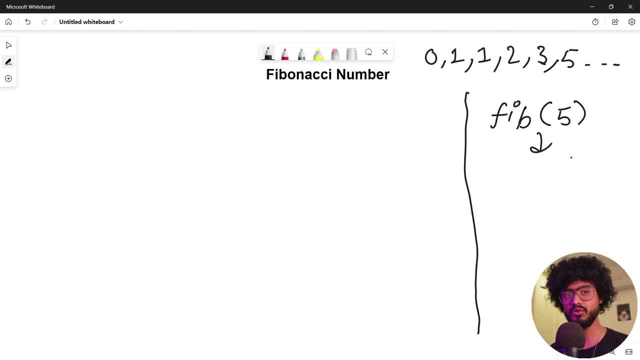 Fib, which takes an input of five. So let's see the rules first. See, as I mentioned, it starts with zero and one, and the index of our array also start from zero and one right. So what are we going to simply say? 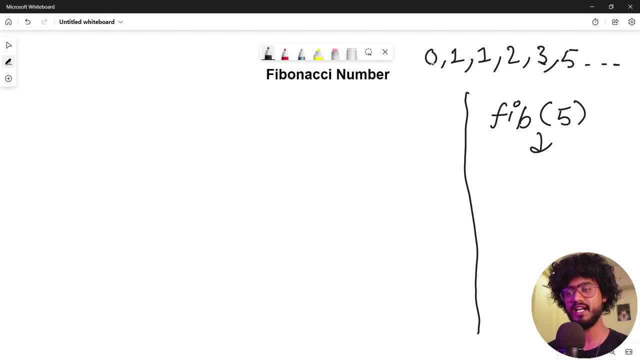 We're going to say, if the input that is provided to us, if it's either zero or if it's one, if it's index zero or if it's index one, then we're going to simply say: return that. So I will say if, and we're considering, and in this case. so let me just remove this. 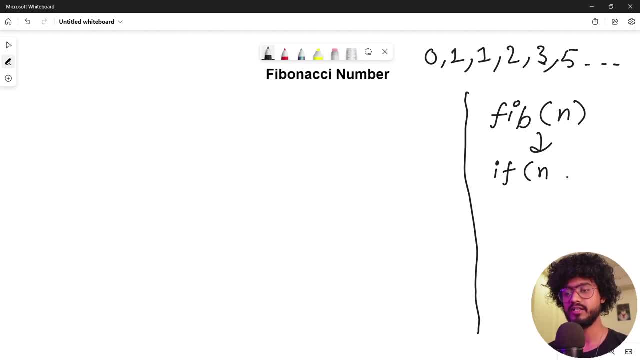 Okay, I'm just going to write an over here. So if n is less than or equals to one, that is, if it's one or if it's zero, then obviously we're going to return and right, Simple enough. But if that is not the case, what are we going to do? 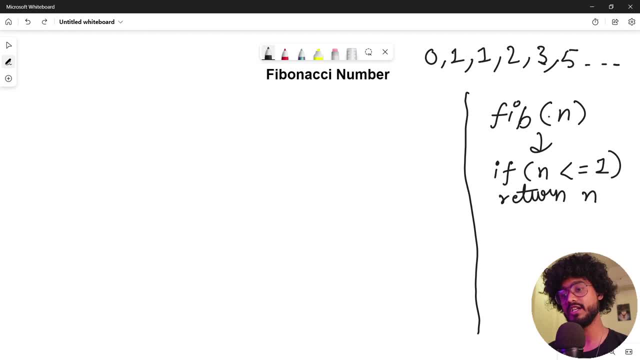 We're going to call this function again, but this time let's say, if our original number was five, if you want to calculate the fifth position. So for fifth position it's going to be the Fibonacci number that comes before it and the number before that number. 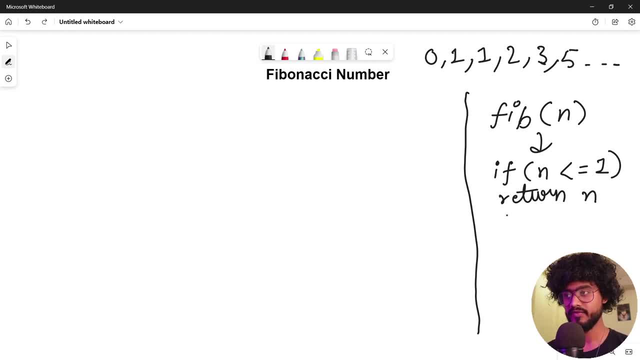 That is the sum of previous two numbers. So what do I mean by that? Okay, If that is not the case, we're going to say else: return What is the Fibonacci number of n minus one and add it with the Fibonacci number of n. 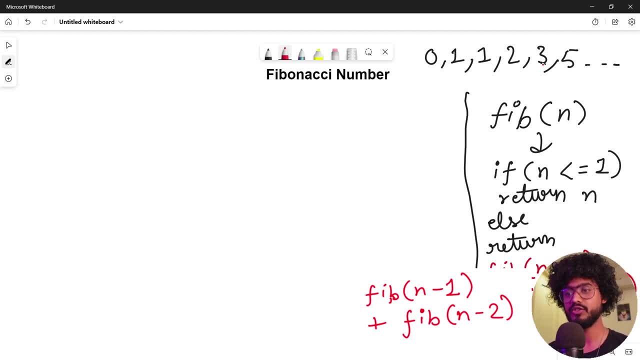 minus two. That's the logic, right? If you're supposed to calculate this position right? Fifth position, then you need to know only the previous two. That's it. You just need to know the previous two and you'll be good to go. 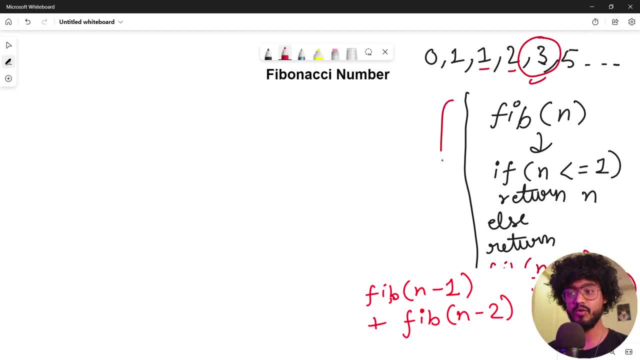 You can calculate this. So that is all we are going to do And this is what our algorithm is going to be. It's that simple. Let me explain you guys with much, much easier visual approach. So okay, over here we have a Fibonacci number function with five as an input. 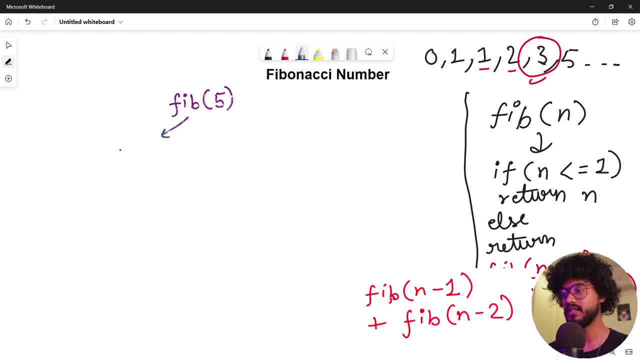 So what we want to do to calculate five, we just need to calculate the Fibonacci number of four, That is n minus one, And Fibonacci Number of Three, That is n minus two. Simple as that, Yep. Now we need to calculate the Fibonacci number of four. over here, 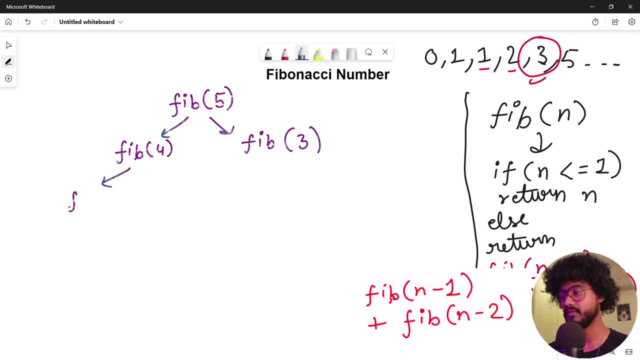 So how do we do that? Again same thing: We need to calculate the Fibonacci number of three and the Fibonacci number of two. Simple as that, Same with here: Fibonacci number of two and n Fibonacci number of one. Let me just write this out: 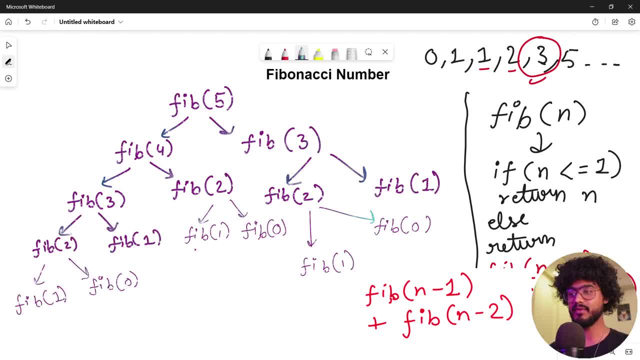 Same for this one as well. All right, cool. So there it is. There's the table. I know my handwriting sucks, but please forgive me for that. So let's see. Let's see what's going on over here. On all of these cases, we have reached our base cases. 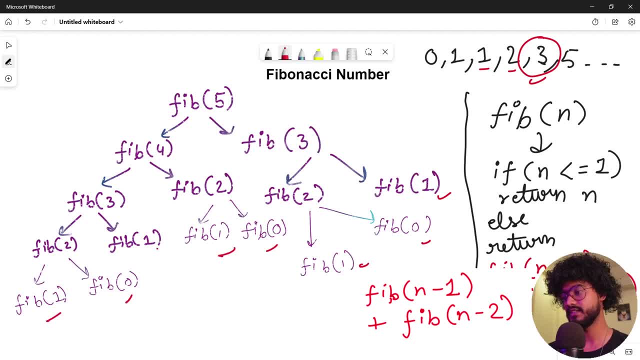 This is our base case: This, this, this, this, this, this and this as well. So our base case is: if n less than or equals to one, just return n. Okay, So this is one That is less than or equals to one. 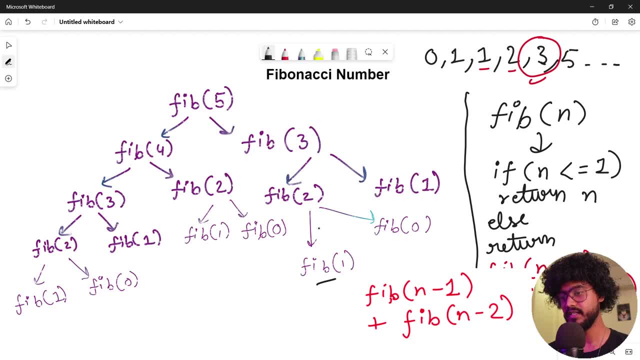 This is zero, Less than or equals to one. Okay, So this function over here will return one. This function over here will return zero. This function over here will return one. This one zero one. one zero one. 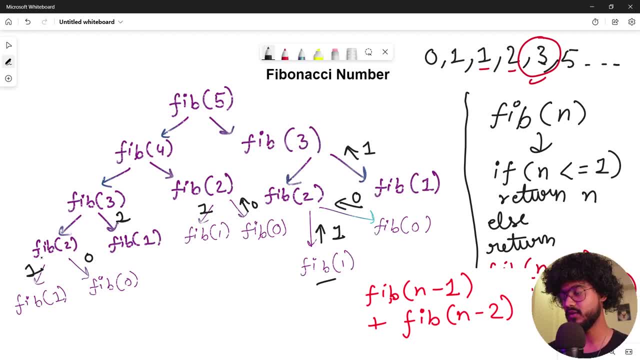 Cool, Now that it has returned all of these base cases. now what's going to happen over here? We know we need to add both of these. So to calculate Fibonacci number of two, we need to add this Plus this, As you can see over here. 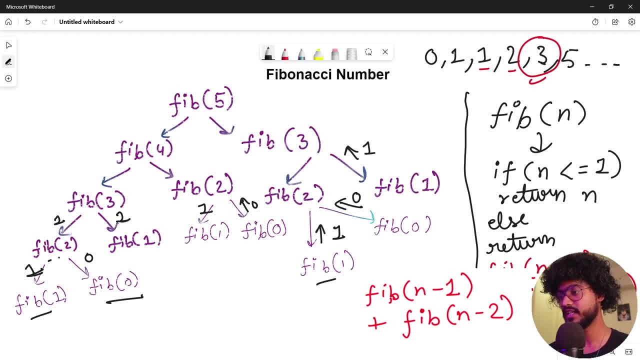 So one plus zero is going to be one. So this function right here is going to return one. So where else is Fibonacci two? Okay, This will also return one. This will also return one, And yeah, I think that's it. 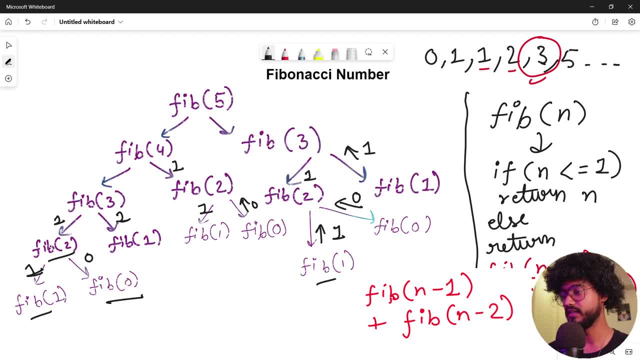 Okay, Cool, Now let's focus on this part. Fibonacci number of three: We know the result of this. We know the result of this: One plus one, two. So we're going to return two over here. Okay, One plus zero one. 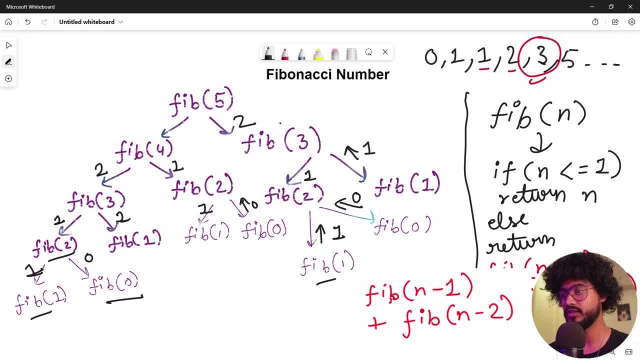 We already calculated that over here: One plus one, two, So this is going to return two. In the case of Fibonacci, number of four, we're going to return two plus one, That is three, And finally, three plus two is going to be five. 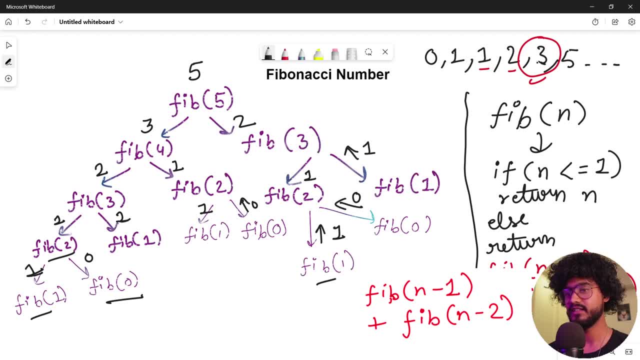 So Fibonacci number of five will be five. Apologies, I mentioned that Fibonacci number of five will be three. That is not going to be the case, since we start counting from zero. So zero one, two, three, four, five. So this is what is going to be Fibonacci number of five. 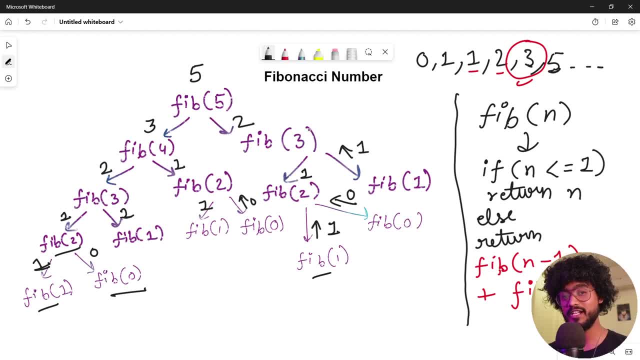 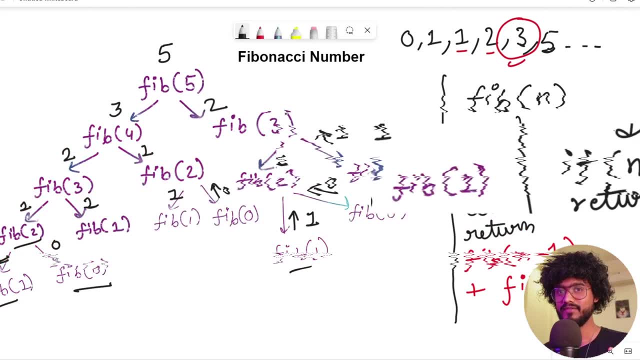 So that is what Fibonacci number is all about. I hope you like my explanation. If you did Hit that like button right now, and I will see you in some time with the explanation of some other algorithm. This guy man, he always interrupts my videos. 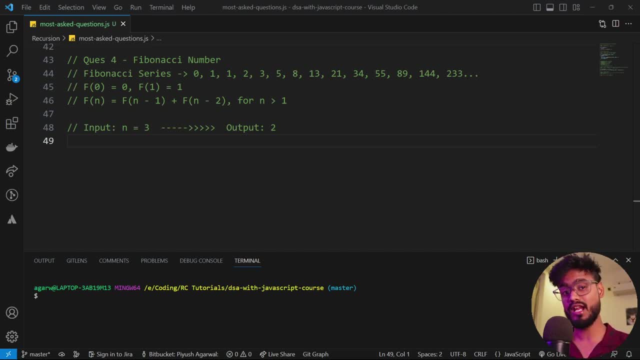 If it weren't for you guys, if you guys weren't liking the way he explains, I wouldn't allow him on my channel. Anyways, let's move on, And I'm going to now write the code for this explanation. But first, before moving on to writing the code for the recursive approach, I'm going 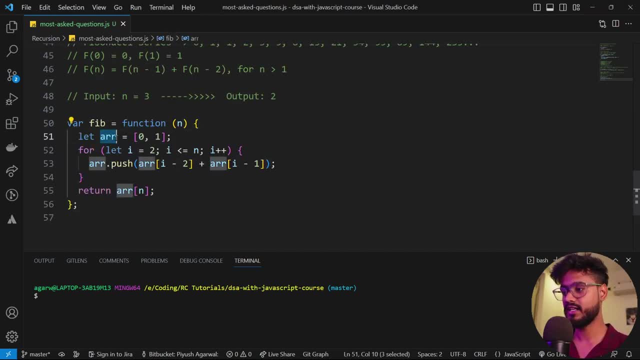 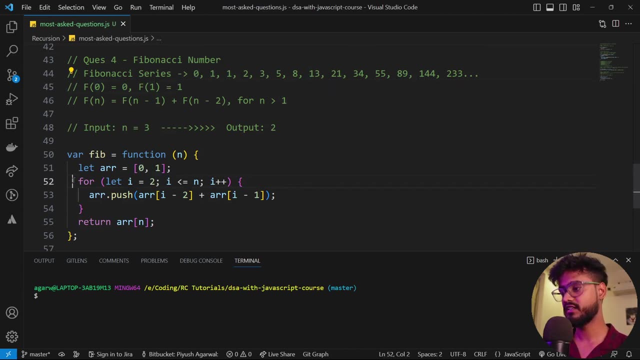 to show you how you can do it by using just for loops. So first we have taken an array, ARR, with initial values of zero And one, because obviously we start from zero, and one right, And then we're going to run a for loop from i equals two, because we already have zero. 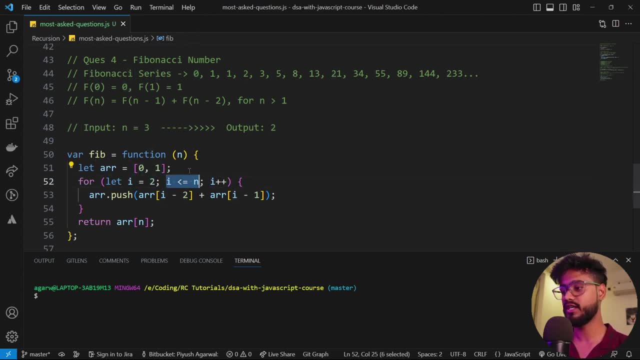 and one, right. So we're going to start from two and we're going to go to all the way to n. So as we traverse further, if the i is two, we're going to say array i minus two plus array i minus one, that is, adding previous both values, right? 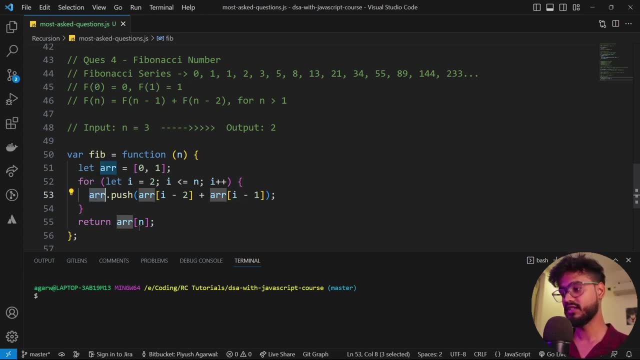 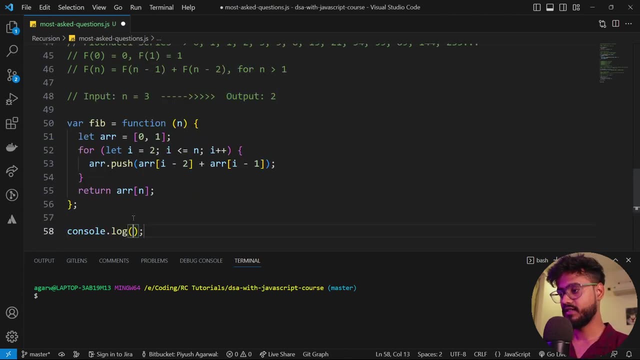 And this is how we're going to populate our array with all of these values And, in the end, if the n is equals to three, we're going to return Whatever is in the third index of that array. So let's find out, and this real quick. 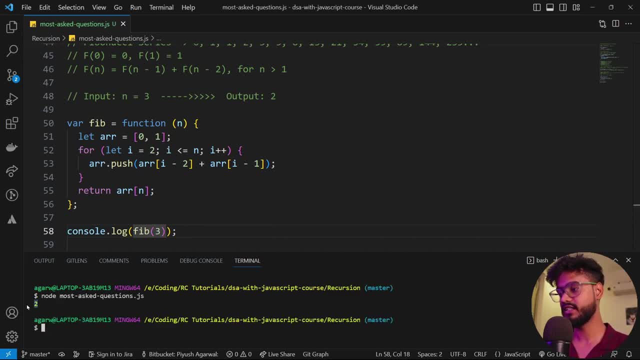 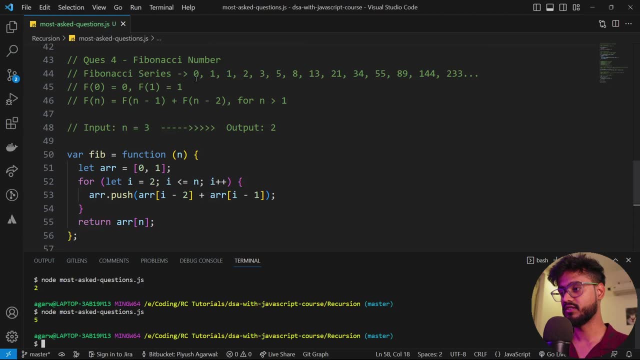 If I say n equals to three and run this, you're going to see we get to over here. if I change to five, let's say then we're going to get five, because in the fifth index that is 12345.. 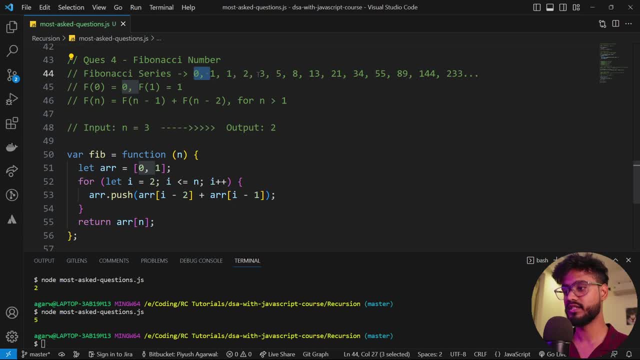 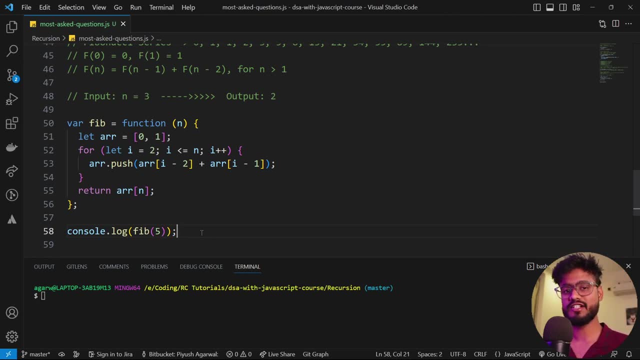 I mean 012345, fifth index. we have five over here, but we're not going to use for loop, right? We're not going to do this. We're going to do this in fashion, boring way. So we're going to use recursion to rewrite this code. 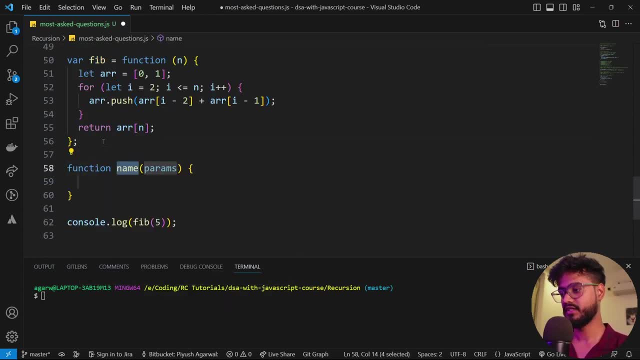 So I'm going to take this function and I'm going to say function fib, recursion, and we're going to take n as an input, And let me just comment this one out for now. All right, so, as explained by algo agarwal, what are you supposed to do, since we already 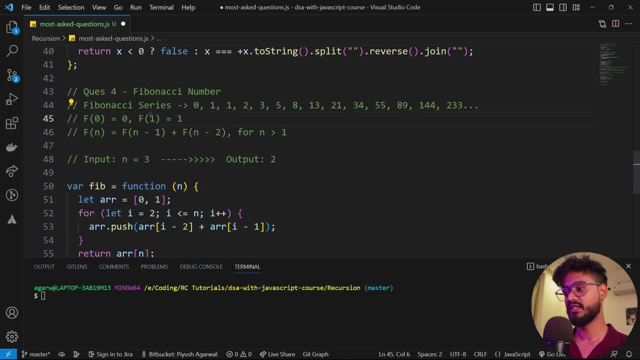 know that if n equals to zero, then it's going to return zero, but if n equals to one, it's going to return one. So we already know what our base case is going to be right. So I'm simply going to say: 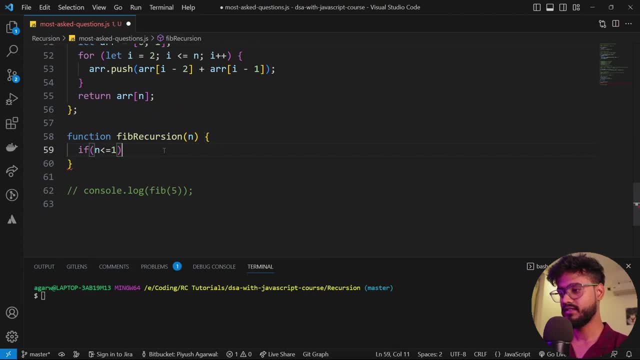 If n is less than or equals to one, then simply return n, Simple right. So that is what our base case is going to be. And now here we're going to branch out this into two different recursions. So I'm going to say: return fib recursion to n minus one plus fib recursion to n minus. 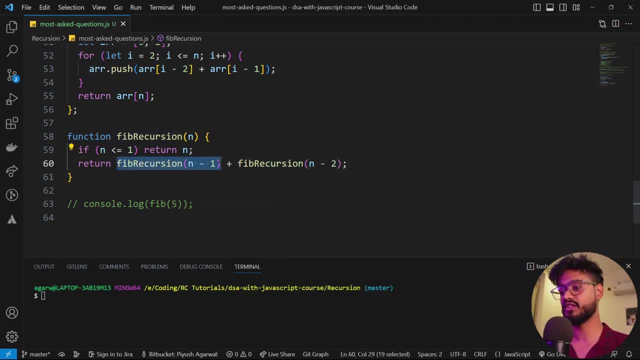 two, And this is going to form that complete tree that you just saw, And in the end it's going to add all of the values together. Okay, Cool, So let me just try to run this recursion and run it, Yep. 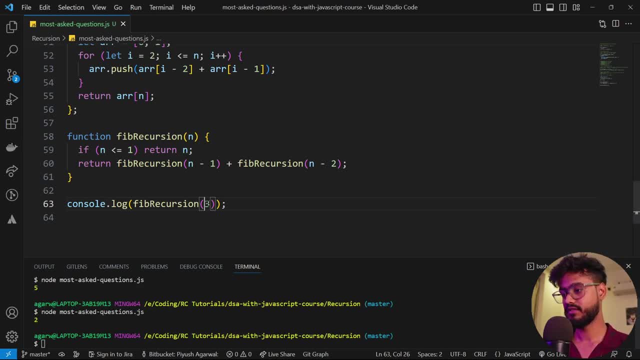 You see, we get five. five, say three, Run it. If we just, you know, add a pretty big value, then it's going to give the result accordingly: Yep, Great. Now let's move on to our next question, which is reversing a string. 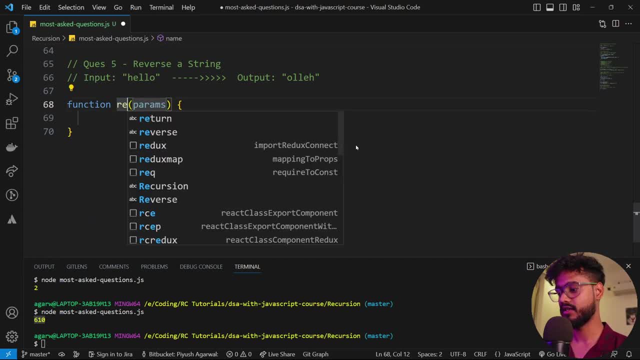 So, again, what I'm going to do, I'm going to take a function over here called reverse string, and this will obviously take a string over here. So what are we supposed to do in this? We're going to input a string and the output is going to be the reverse of that. 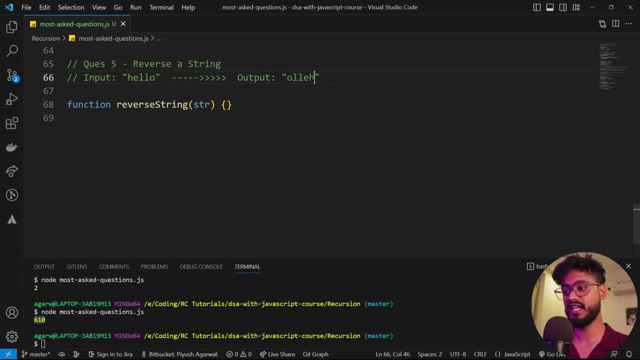 So if it's H E double L O, the output will be O double L E H, right? So obviously, before moving forward in this video, you have to go and try this out yourself first. So I hope you were able to do it. 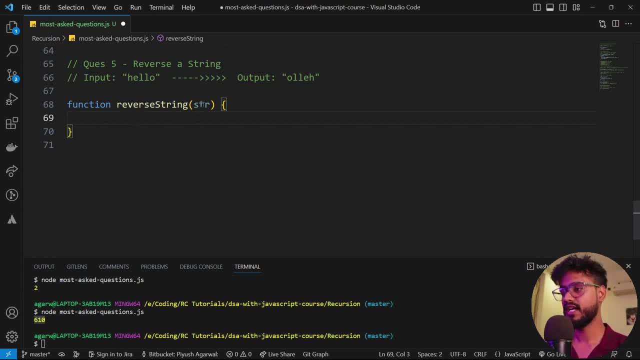 If not, let's see, let's find out how to do it. All, right, So we have a string over here, right? And what are we supposed to do? We're simply supposed to take one character from it at a time and just put it at the back. 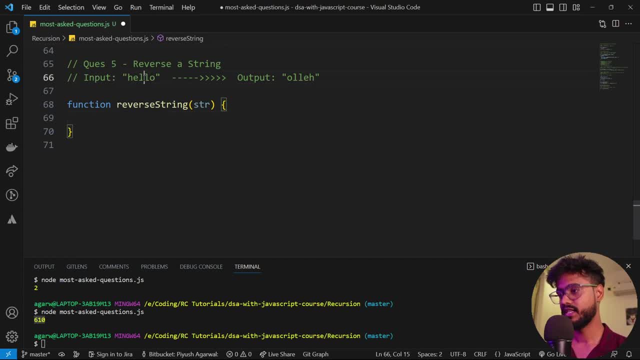 of the string. But we are supposed to do it. We're supposed to do it by using recursion. Okay, So let's say we have hello over here. We can simply take H at once and we can put it over here, right? 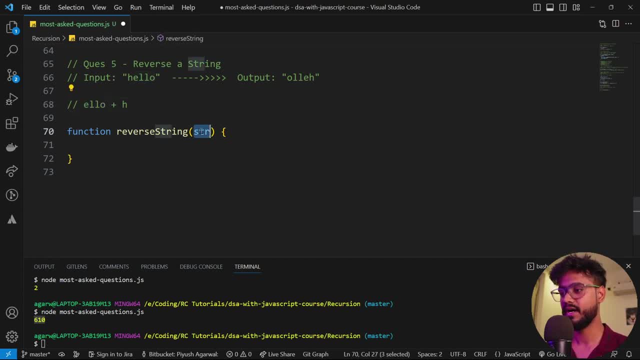 Plus this, and then we can supply this remaining string back to this function, And then it's again going to put the logic that we're going to take the E and just put it over here, right? So how can we do this? Let's see. 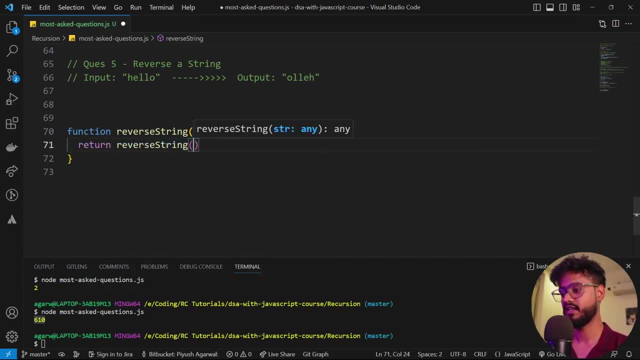 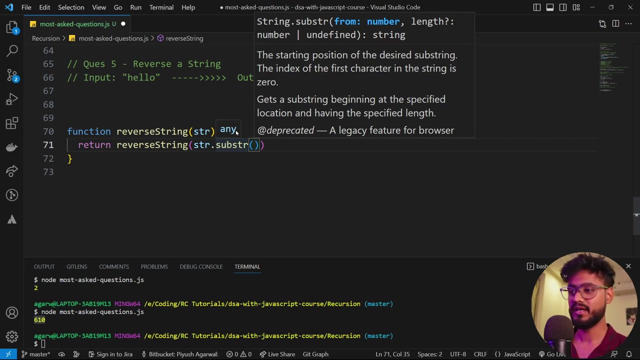 I'm going to say return reverse string. Okay Done, I'm going to simply take the string which was provided to us: dot sub string. Now, you might not be familiar with this functions right now because I haven't made a video on strings yet. but don't worry, that video is going to drop very, very soon, but I'm 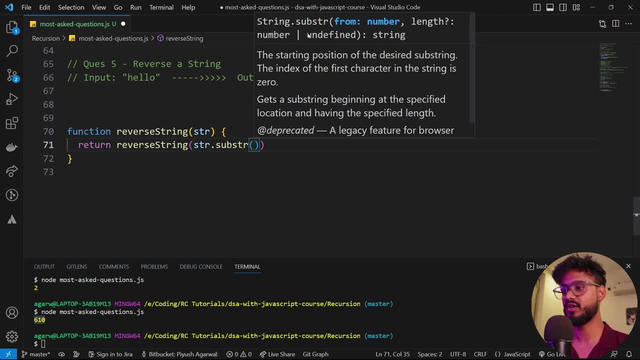 going to explain you what this function does over here, The sub STR function. what it does is we are supposed to provide it a number that is the starting position of the desired substring. So the index of the first character in the substring is zero. 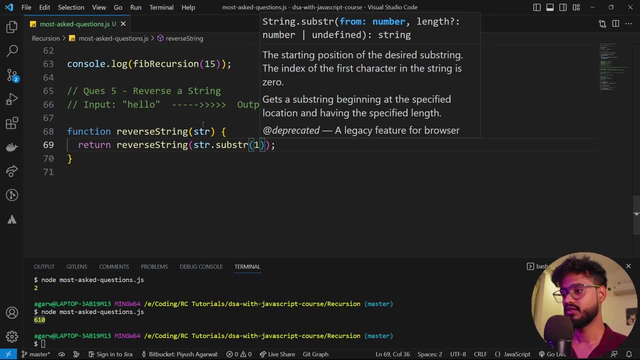 So what it will simply do is, if we provide it, Provide it with one over here. So what you'll do is it'll start from one and it will take the complete string, just like this right. And then what we can do is: we can we have taken this string and then we can put H at. 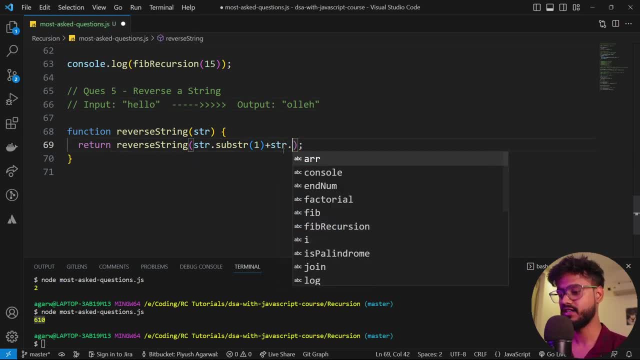 the very last. So we can take the first character now. So I will say STR dot. there's a function called care at. So what carrot does is it returns the character at the specified index. So we need the first index, right. So we're going to say zero. 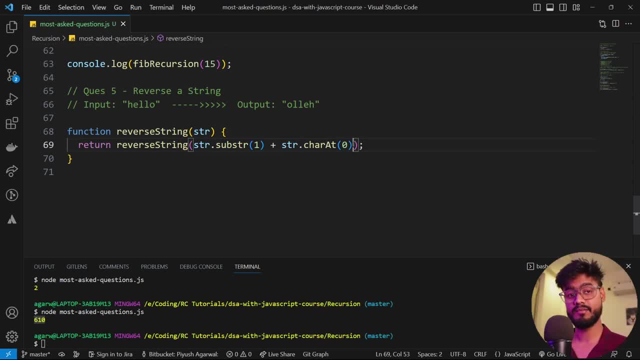 That's it. That is all we were supposed to do, but wait, we haven't written the base case over here yet. So there's going to be one point right where all of the characters of this string will be exhausted and we will be provided with just an empty string. 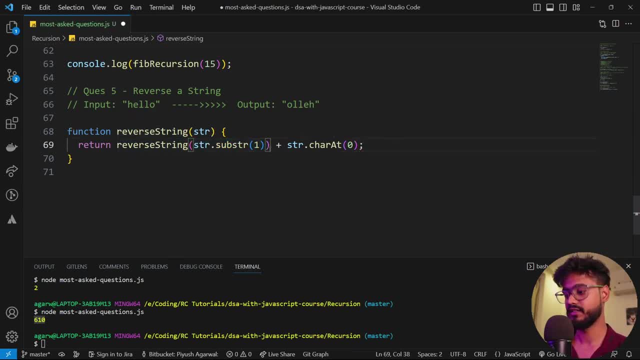 Also hold on. I've just written it inside of this bracket. This is how it's going to be. It's going to be outside of that function. Yeah, So it's gonna at one point exhaust the complete string, right? So we're supposed to say, if STR equals to empty, then we're going to return empty. 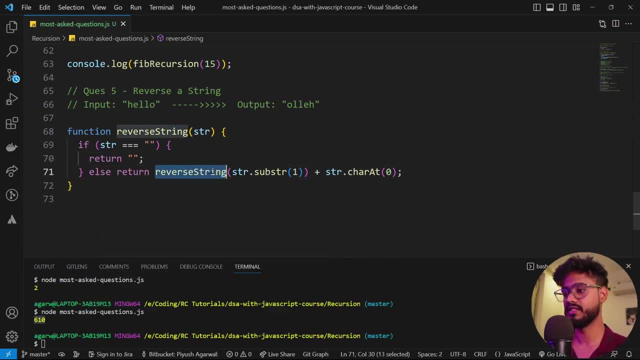 right, Else, We're gonna. We're going to do this over here. Don't worry, I'm going to dry run it as well in just a second. Let me just console log this and run this reverse string. Hello, If I run this, yep, we get the reverse of this string. 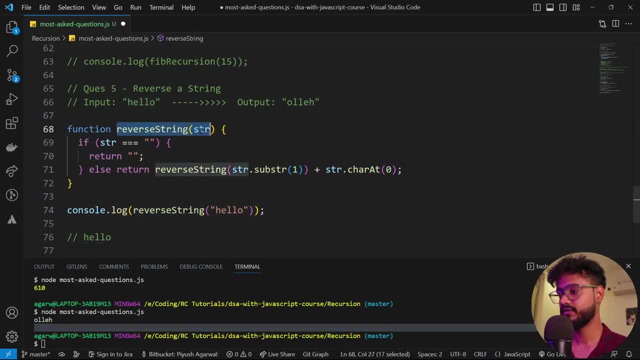 So let's see what's going on over here. So we have this hello over here right In the first iteration. this is hello, Okay. So in the first iteration We're calling this reverse string function starting from the index one. 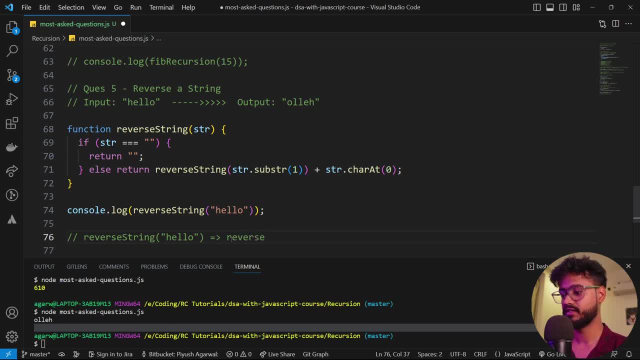 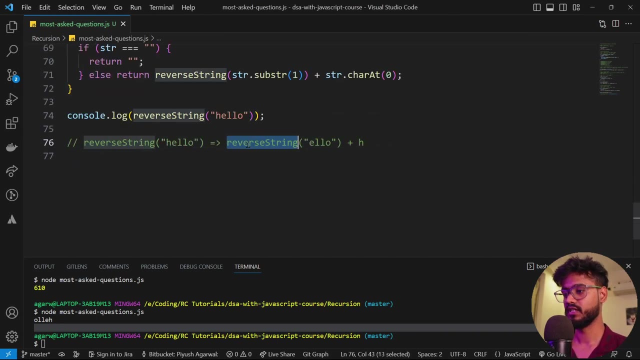 So this will. what this will do is this will call reverse, with reverse string starting from one. So E double L, O right. And then we are adding the first character, which is, in this case, H plus H, right. That is what we're going to do. 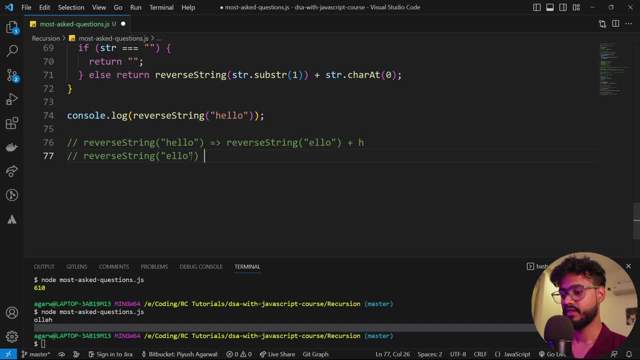 Now let's talk about this. What will this result in? This will result in Starting from index one, So it will be double L, O plus E. right, Similarly for others as well. Let me just drag this out real quick, Yep. 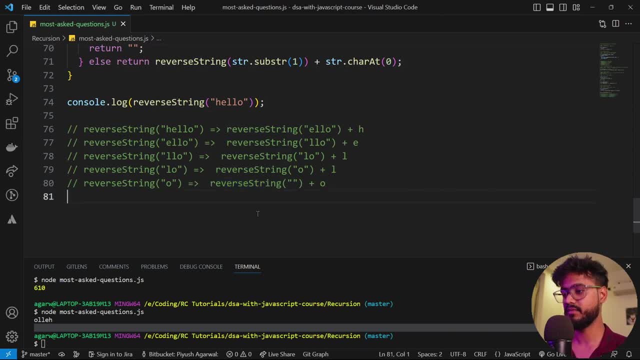 Just like that. So we've reached over here, right, And now we're calling reverse string with the empty string. So when we call it with the empty string, then this is going to return with the empty string, right? Okay, Let's replace it with the empty string. then, right over here. 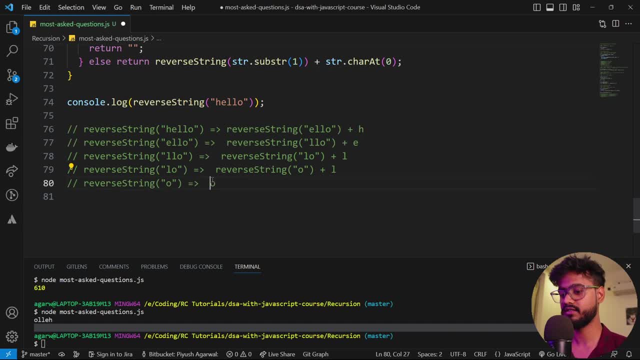 So So empty string plus O will obviously return us. O right, Now this thing is returning us. O Cool, Let's just take it and replace it over here. O right, So O plus L will obviously will be O L right. 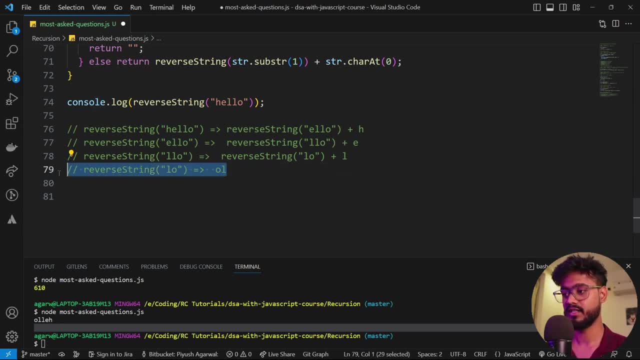 So this L? O is returning us O L. fine, I'm going to remove this and replace it over here. O double L. fine, Let's take it and replace it over here. Let's take this and replace it over there. So you see, this is how you get a reverse string by using recursion. 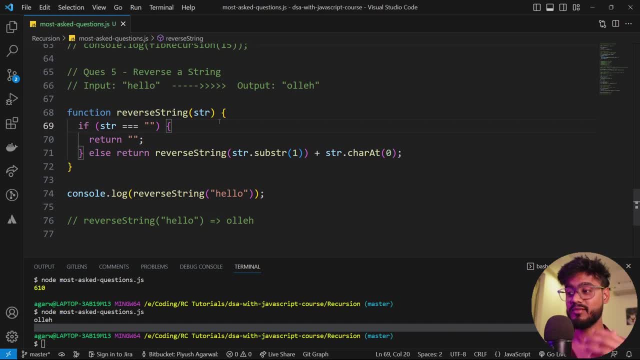 I hope now you must be able to find recursion really easy, right, Because now you're able to think how recursion works. There is a pattern, If you see these questions right, You're supposed to call these functions and there's always going to be a base case. 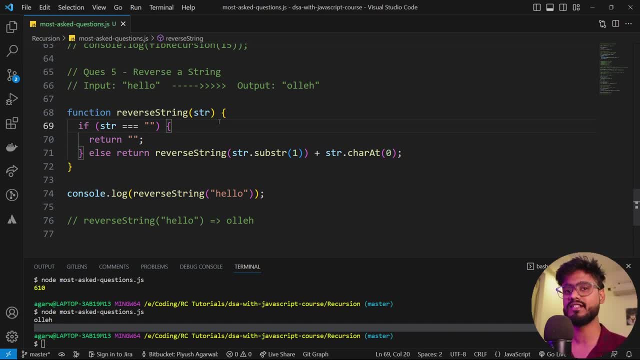 And this base case is usually very obvious. If you just put a little bit of common sense, you're going to understand how easy it is to find the base case. And once you find the base case it's- I think it's pretty much easy to you know. do the recursion based questions? 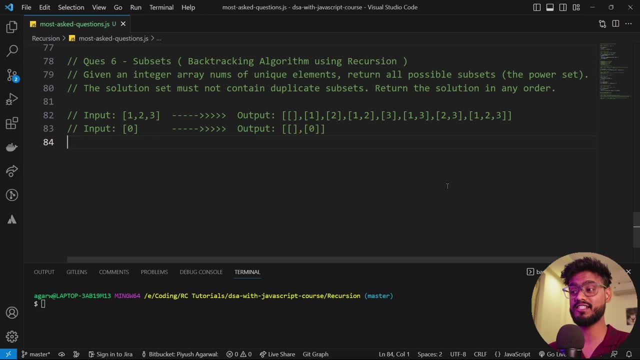 And this next question is called subsets. And, trust me, this has been asked to me multiple times in the past during DSA interviews, So I would need your full focus to understand this problem. So let's see- Also one more thing- that this is an example of what we call a backtracking algorithm. 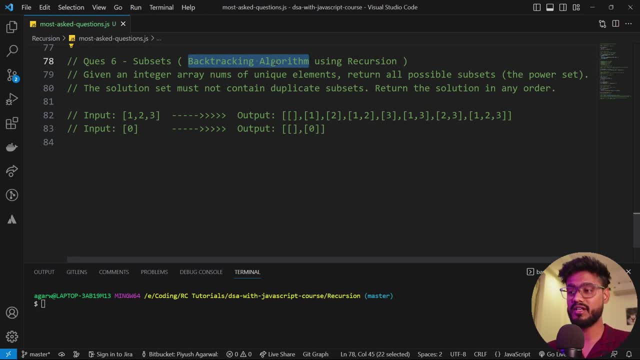 which we're going to talk about in much in depth in our future videos, But for now, you're going to get a brief understanding of what backtracking algorithm is and how you can implement it using recursion. So So we've been given an integer array, nums of unique elements. 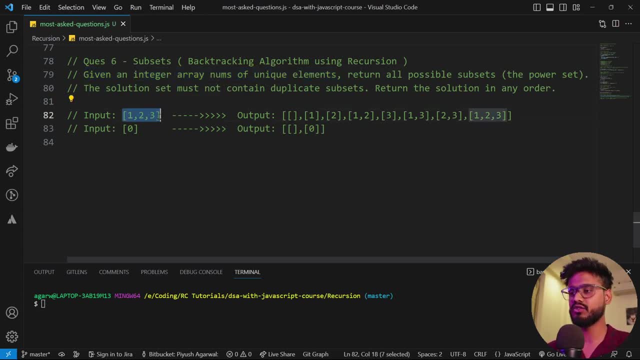 So we're going to have a array just like this, with unique element, that is, no element will duplicate itself, Right? So we're supposed to return all of the possible subsets. That is the power set. Now, what is the power set? So we have this array over here as an output and this will contain all of the possible. 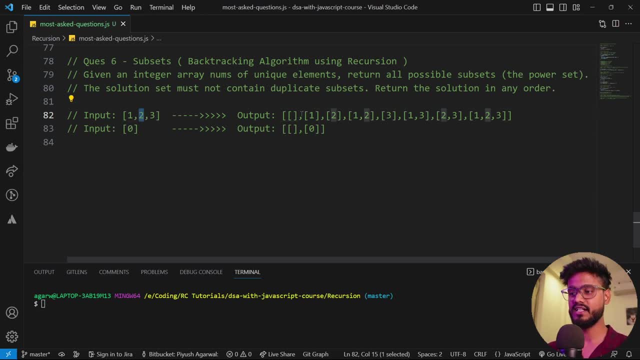 combinations that this particular numbers can create. So, as you can see, we can either create a combination of an empty array or we can have one, two, three. One, two, three, one three, two, three. one, two, three. 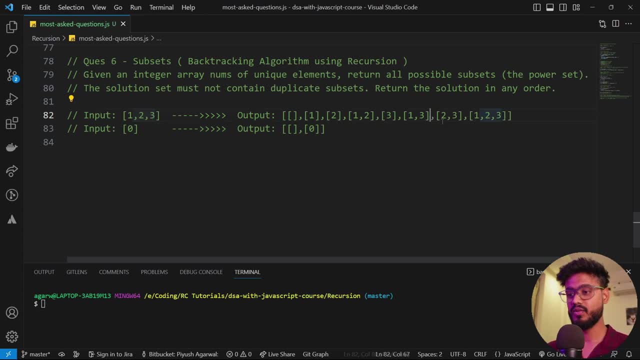 So these are all possible combinations. Now keep one thing in mind: one comma three and three comma one are absolutely same. So it doesn't matter The sequence, doesn't matter if both of the numbers exist or, you know, if the unique number exists in a single array. 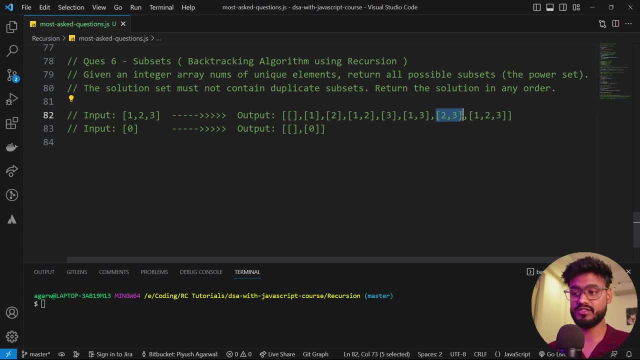 So don't think two comma three and three comma two as separate entities, because they're the same. So that is why the solution set must not contain the duplicate subsets. It should contain only the unique subsets And also solution can be returned in any single order. 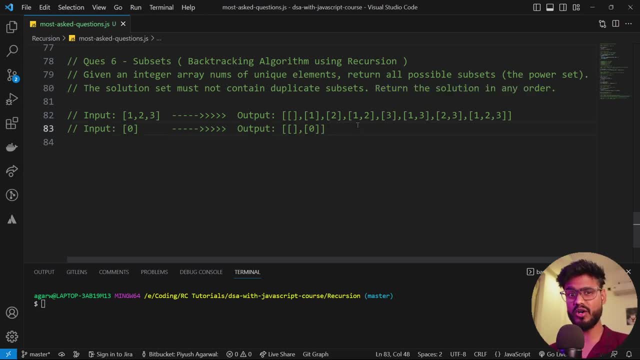 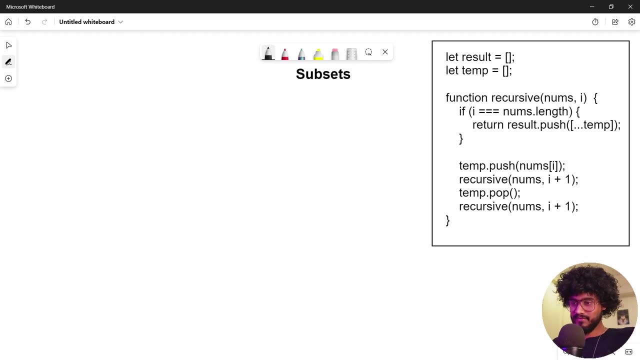 So let's try to first understand this problem in a visual format- And no, I'm not giving you Algo Agarwal this time. I'm going to explain you this in a visual format. Yep, Algo Agarwal is back. 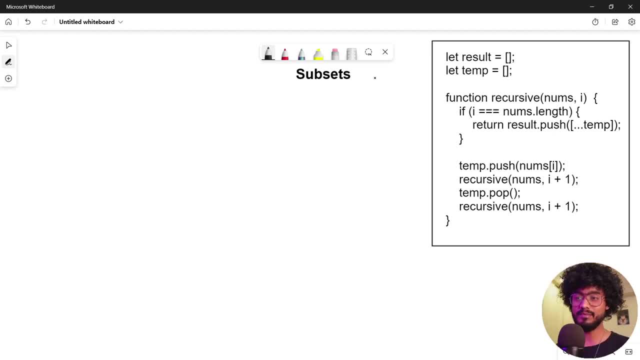 Let's continue. So let me explain you how you can efficiently write this subsets algorithm and let me explain you visually how this is going to work, because this is a pretty complex algorithm and you need an expert like me to explain you, Not some noob like roadside coder. 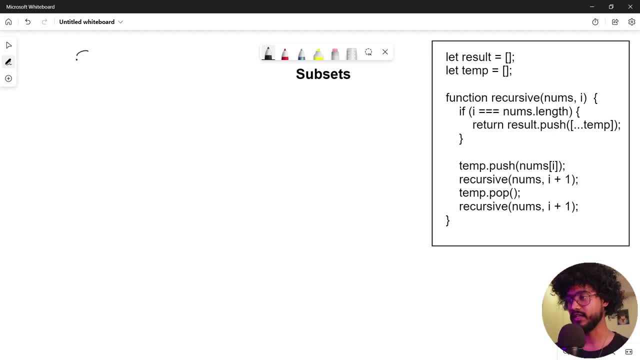 All right, OK, cool, Let's get started. So we have been given an array over here, Right, Let's say we can say it's one, two and three And we are supposed to generate the all possible combinations of this array. 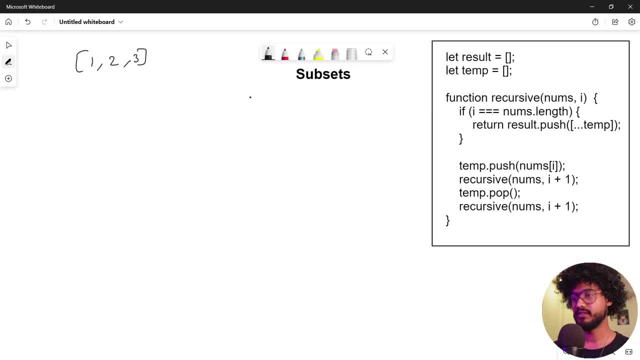 That is all possible subsets that this array can create. Right, So let's see what is the approach that we are going to take. So we are going to take two global variables: First, the result, and other is the temporary variable, or the temp array. 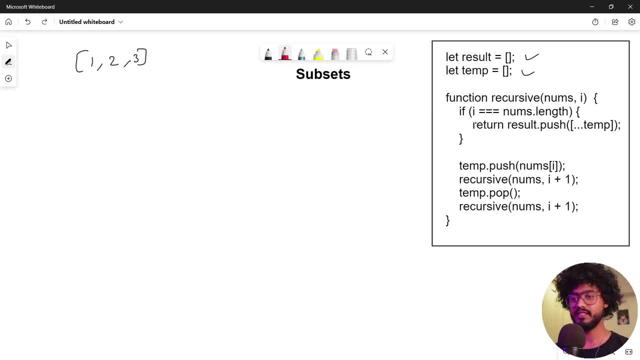 And then we have this function called recursive. Now, instead of this, the approach that we are going to take is this: So, by default, we have an empty temp array. OK, so we're going to take an empty temp array over here. 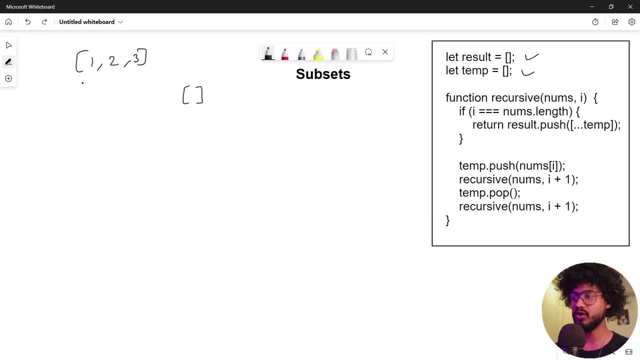 Fine, So now what the approach that we're going to take is now, amongst all of these three, to create a subset. either a subset can include one or it cannot include one Right. Similarly, either it can include two or it cannot. It can include three or it cannot. 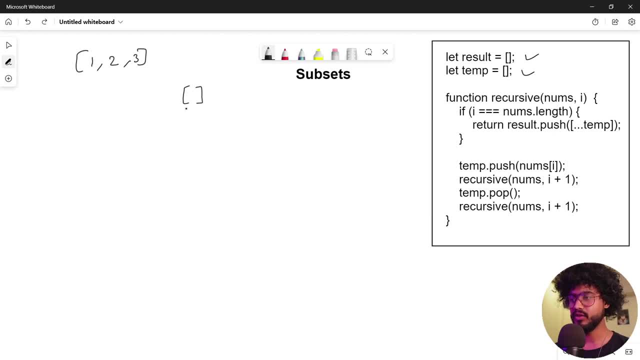 Right. So that is exactly what we're going to do every time We're going to make two recursive calls. In one recursive call we're going to say, OK, take one, But in the other one we're going to say, no, don't take one. 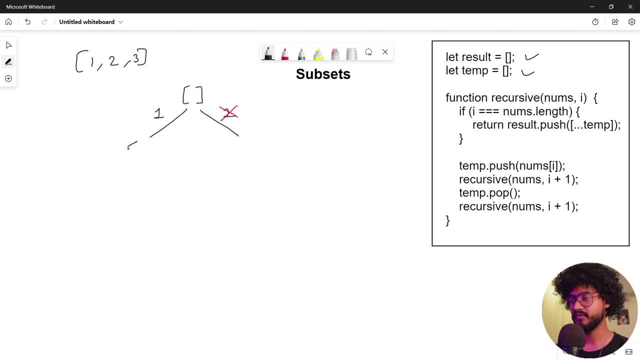 So let's say, to create our first subarray, we're going to say: take one. So we have added one into this array, Fine, And the other array remains empty. Cool, Now. similarly, we are going to do for two as well. 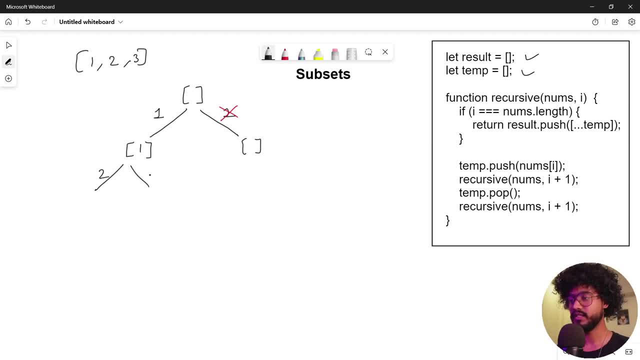 For all of these, we can either take two or we cannot take two, Right? So now our array contains one, One, two, And this array doesn't contain two, So it's just one. Similarly, here as well, it can either take two or it will not take two. 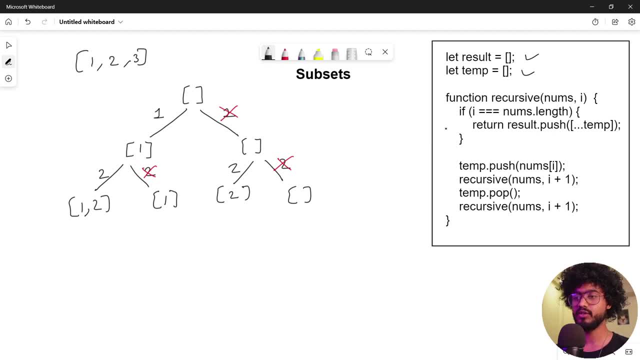 And it remains empty. So, if you notice, in our algorithm that is exactly what we are going to do. So we have this recursive function which take nums and I, and we have this base case too. OK, let's not talk about the base case over here first. 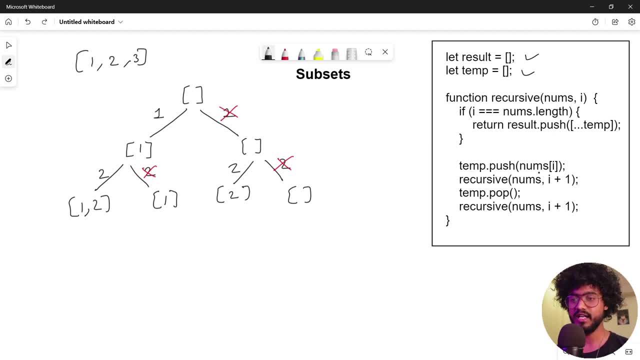 In the temporary array Right, We are first going to push the current values, That is, the current value of I. So when we call this function right- So OK, I haven't written that- when we call this function for the first time with the 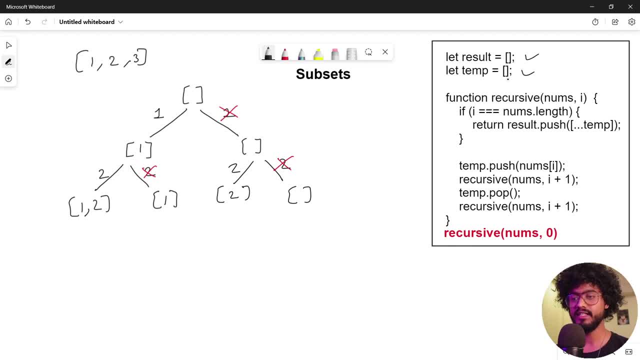 nums array and the zero as the default value. So here in the temporary array we're going to say temppush nums of I. So nums of I is one Right. So, as mentioned, either we can take one or we can not take one. 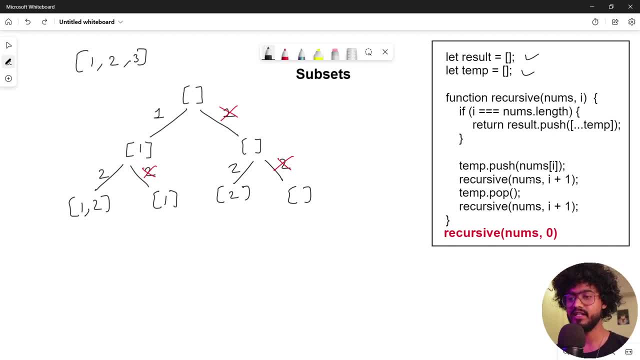 So I'm going to first say: just take one and push it to this temporary array and just call this again. So if you see, over here We are calling this function again. This right over here is basically our function that is being called, but with a new array. 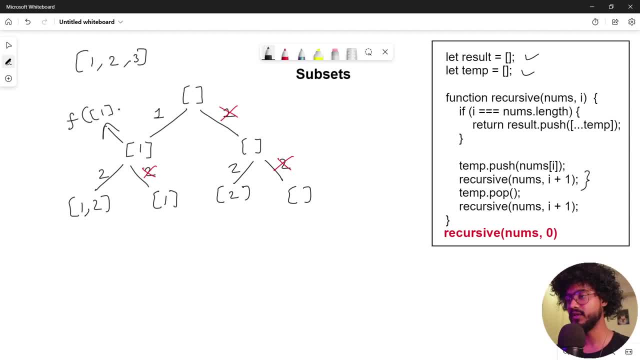 called temp, And right now, temp contains only one and the updated value of I that is one. Now, why did we do this? Why did we do I plus one so that we can move to the next element. So we have already taken one right. 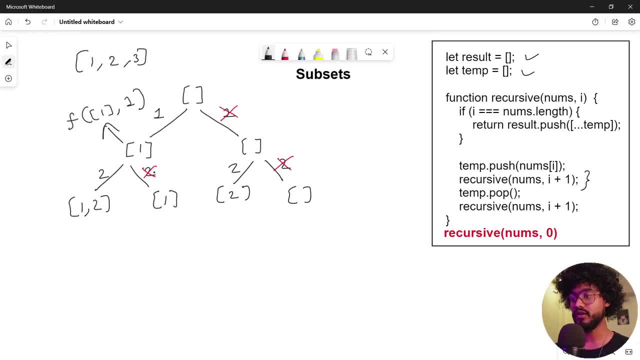 We don't need to operate on one anymore. Now we need to take two or we need to reject two. So again in the next iteration We're again Going to do the same, But if you see below this we're doing temppop, that is, we are rejecting one. 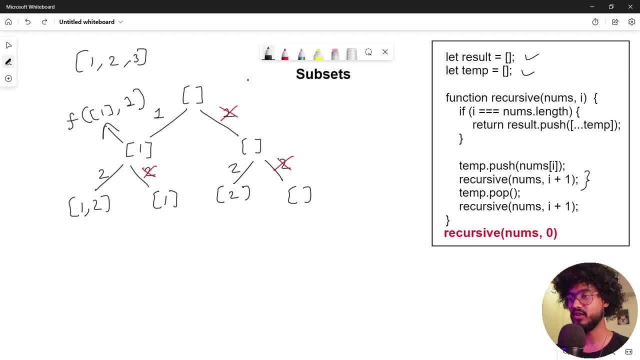 So in this one we just added: So temp in the first case was this over here, but temp in the second case, that is temppop. So we removed the element from the temp. So now temp is empty And now we are sending an empty array to this recursion. 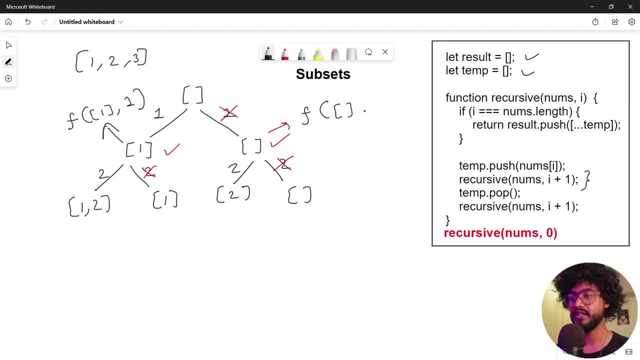 So this right over here will be F of empty array and I plus one, that is one over here. Now, if you Call this function again, you're going to go back. you're going to say temppush nums of I. Now we are pushing the current I. 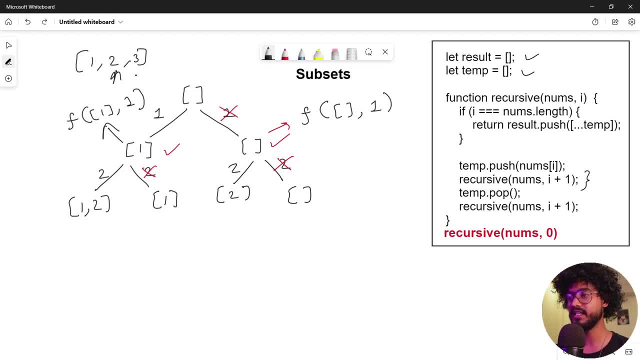 So what is the current I One and what is one? One is the index of two. So we are pushing one inside of this temp. So now you can see, we can either take two, We are taking two inside of it. So our array will look something like: 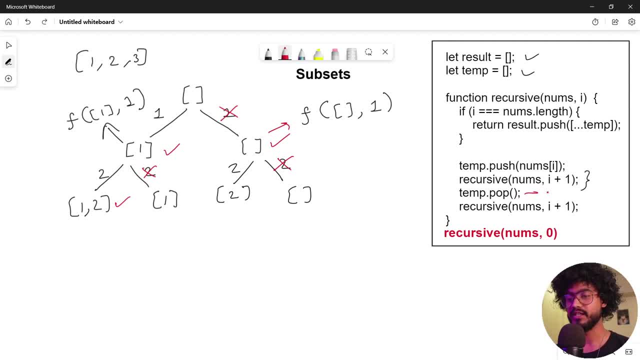 This, or we can either reject two, that is, we are popping the two from the array, So we are removing the two. In this case, our array will look something like this: Again, we are going to make the same function, calling both of the cases similarly in this. 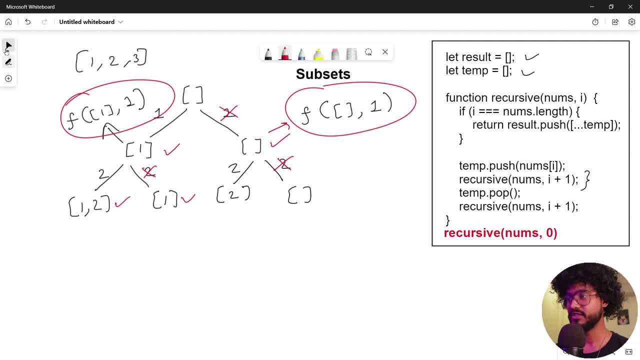 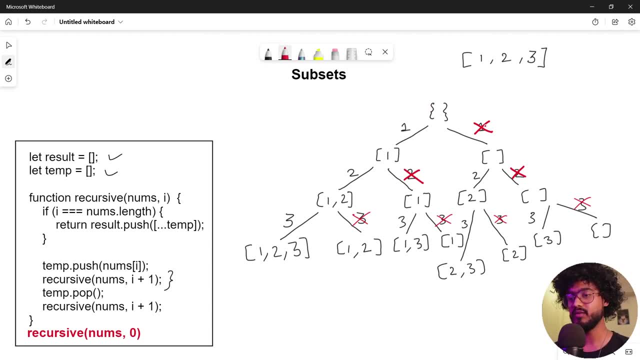 recursive call as well. So I've actually written this completely. Let me just show you. Yeah, there it is. I've written this complete diagram over here. So in the first iteration we are either taking one or we are rejecting one. 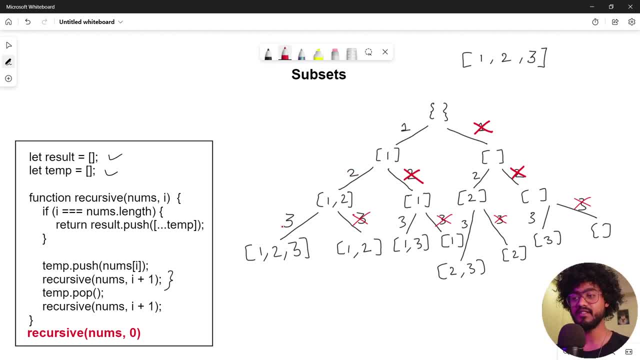 And this iteration as well. either we are taking two or rejecting two. In this iteration as well, we are either taking three or rejecting three. right, And that is what we are going to do for all of these, And in the end, you're going to see, we get all of these final elements. 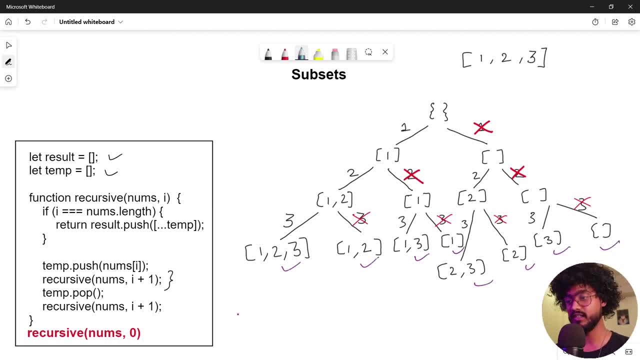 As our answer. So this is what our answer will look like This right over here. You can tally this with all of these results and you're going to find this exactly the same. We haven't yet discussed the base case. So when we happen to reach this condition, that is, I is equal to n, because we are increasing. 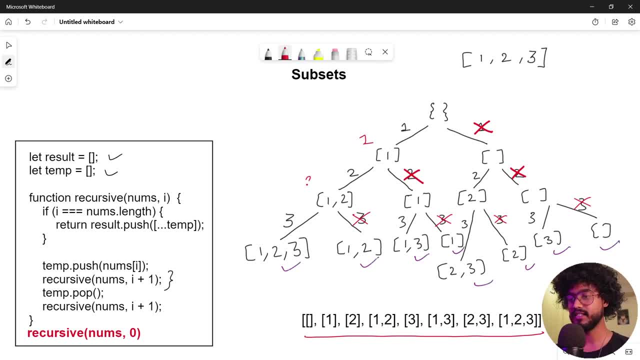 length of I every time right. In this case I is one. In this case I is two. In this case I is three. So as soon as we reach the length of the array, that is, when I is equal to nums dot length. 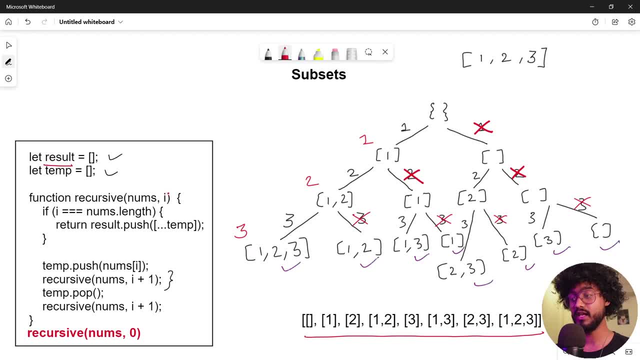 we're going to say We're going to take this, This result array, that is the global array. We're going to push whatever we have currently in temp. So currently we had one, two, three, So we're going to push that inside of this result array. 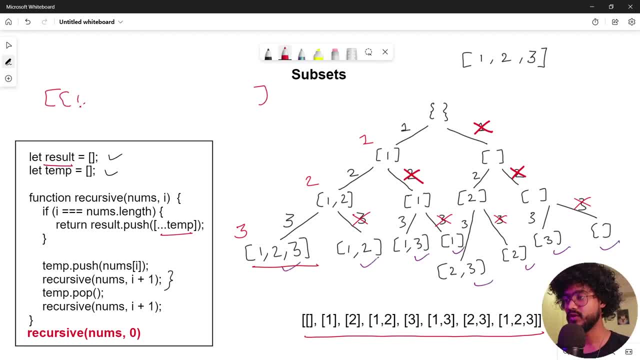 So this is the, let's say, our result array, And we first pushed one comma two, comma three, Then again we're going to push one comma two and so on with all of these array over here, And then it's going to give us this final result. 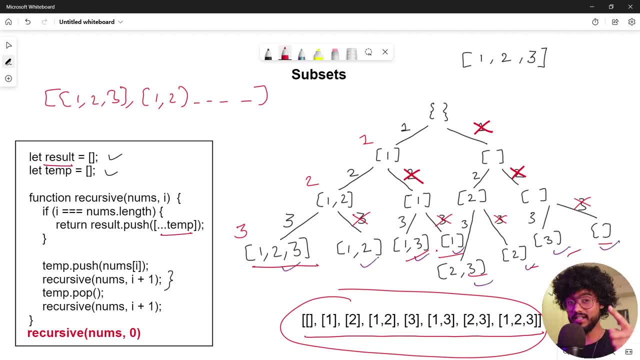 So, yeah, awesome. I hope you like this explanation again. If you haven't yet subscribed to the channel, hit that subscribe button right now. And don't forget: Algo Agarwal needs to write code as well. So open your Instagram app right now and search roadside coder and message him to give Algo. 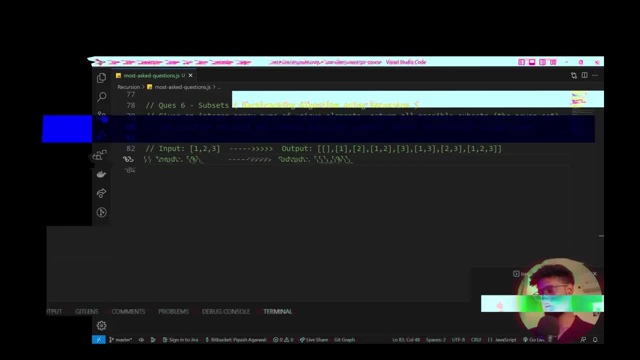 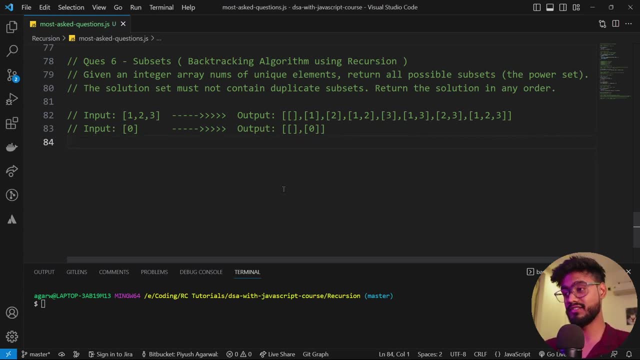 Agarwal opportunity to write code as well. Oh man, not again. Anyways, I'm just going to go on and continue to explain you the code. now, since you already got an overview of- you know, high-level overview of the code, let me just quickly write that. 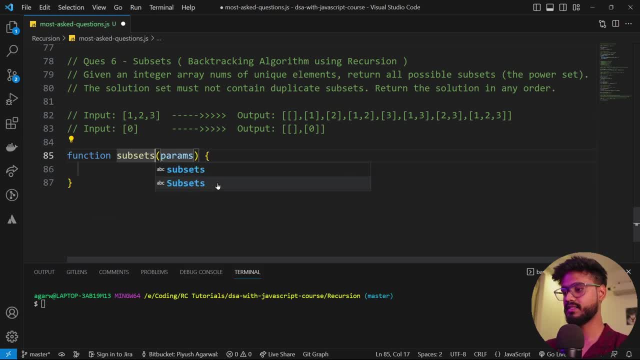 code down. So I'm going to get a function over here called sub sets And, as explained, it's going to Take an array or called nums. Now we're going to take a few variables. First fall is going to be result. 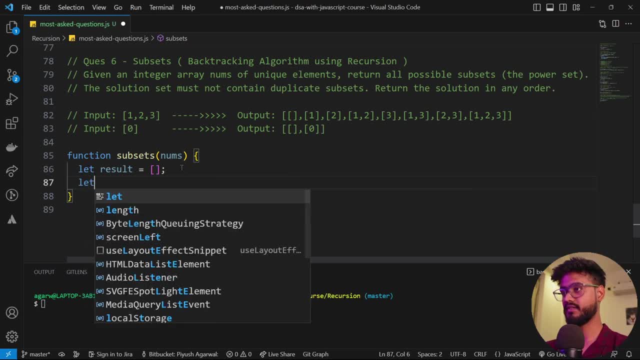 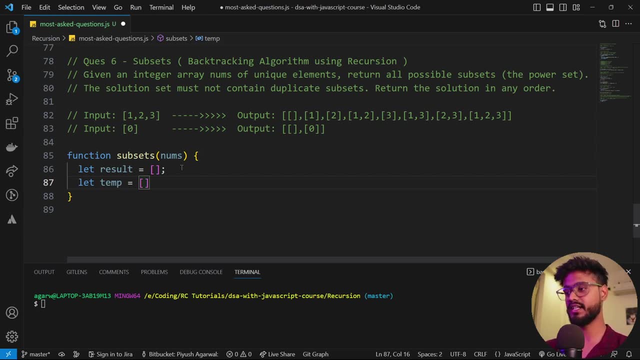 Result will be an empty array. Then we're going to have temp, which contain, which will contain, the temporary elements of this array, That is, the subsets of this array, And then we're going to, you know, keep on changing the temp. 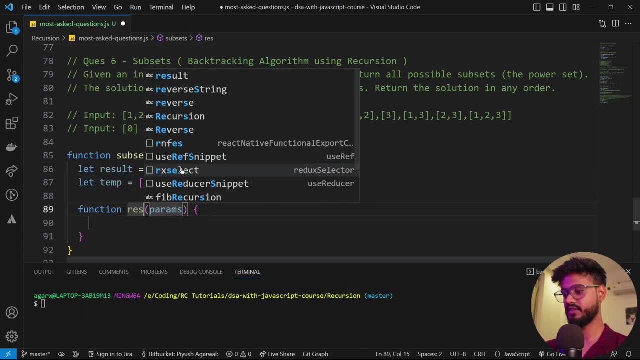 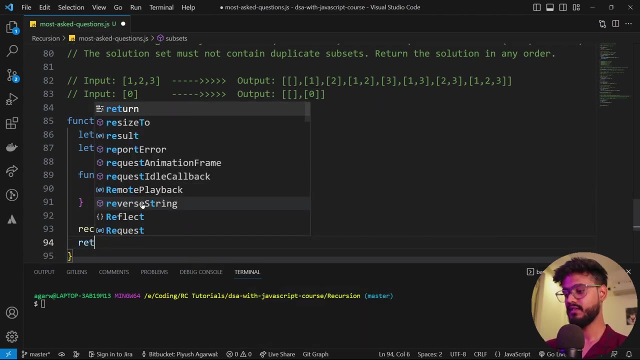 Now, next, we're going to create a function called I don't know, let's say recursive subsets, And this will take nums and I, and in the end we're just going to execute that function- nums, comma, I- and return the result. 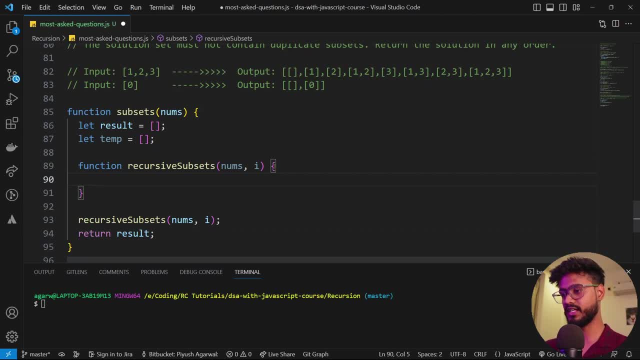 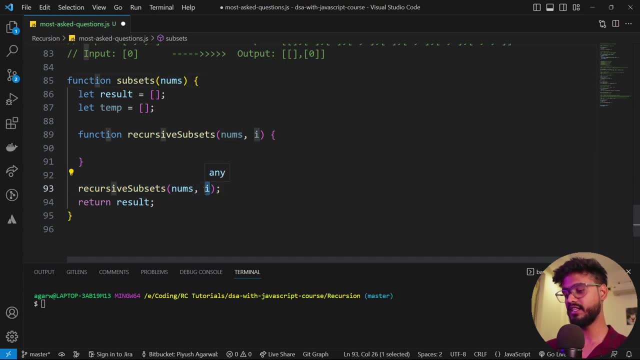 Don't worry, I'm going to explain everything step by step. So let's go inside of it. So we're going to start this by using our nums, That is our array over here, And the initial value will be zero, because that is where we are going to start. 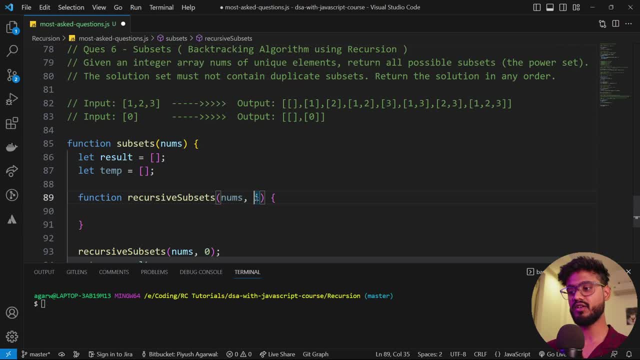 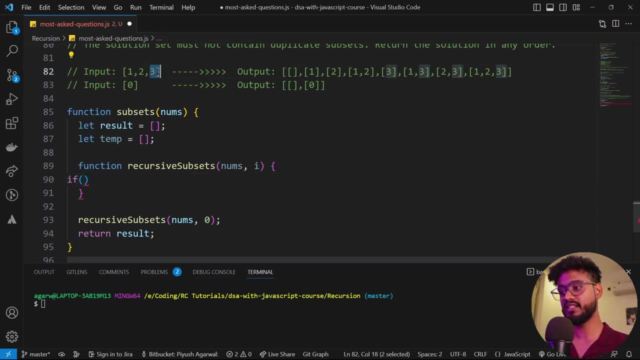 We're going to start from the first index, right? So we have provided the initial value of I as zero. Now let's just first get the base case out of the way. So simply, I'm just going to say: if it reaches the very end of the array, then we're going. 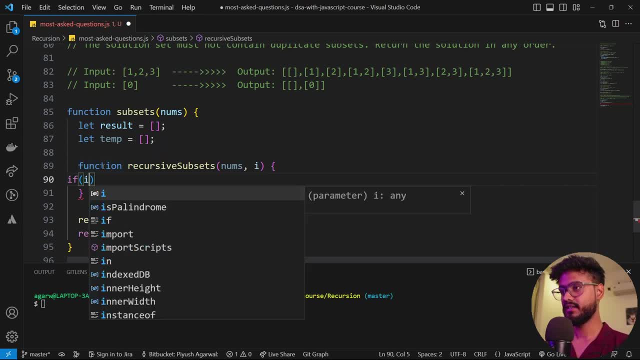 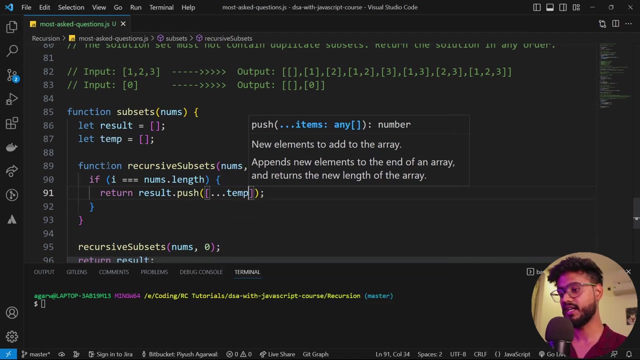 to return the result, right. So I'm just going to say, if I is equals to nums, dot length, that if it reached the length of the array, then simply return result, dot push and whatever we have inside of our temp array. So our strategy was this.